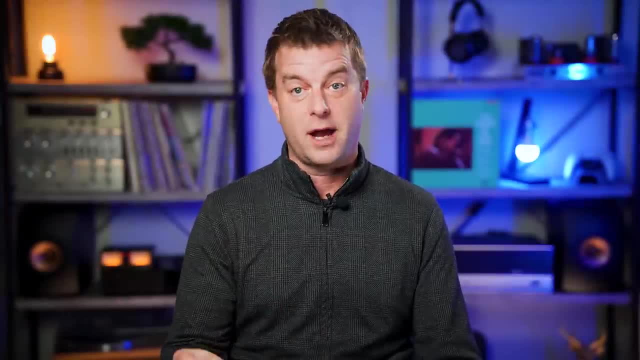 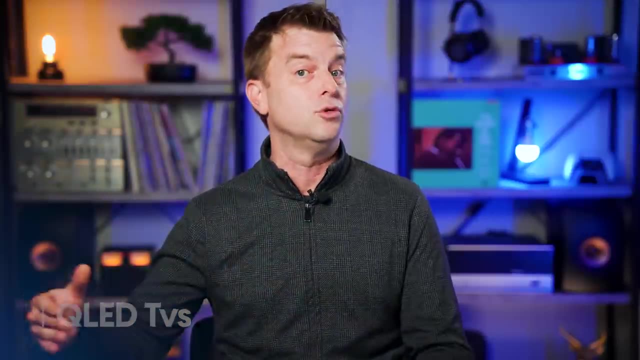 my personal favorites. These are the TVs that I recommend to my friends and family. Sound good? All right, let's get into it. I want to start with the QLED TVs and then we'll migrate to OLED TVs. Now, if you're not familiar with the difference between QLED and OLED, I've got a video for that. 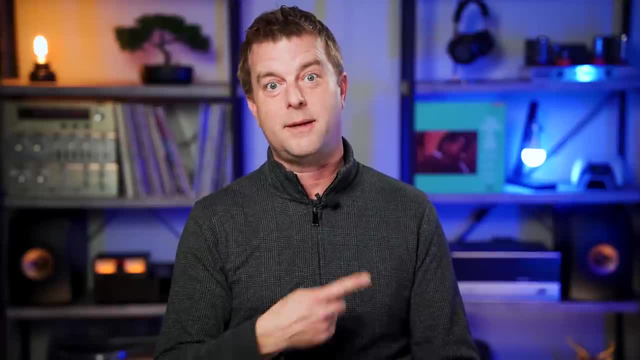 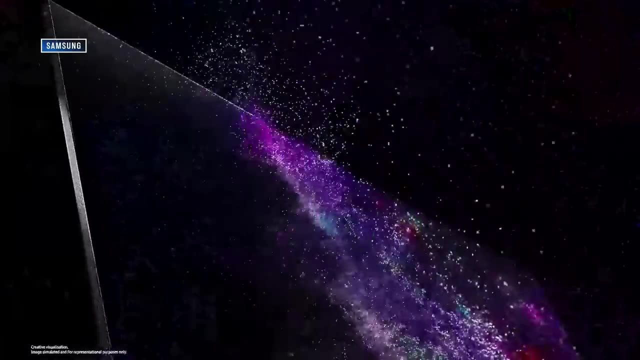 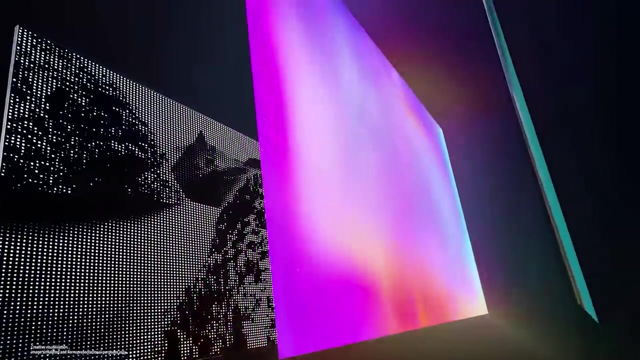 again linked down in the description, and it's probably popping up over my left shoulder right now. Yeah, see, there it is, But here's the short version for you. QLED TVs are LCD TVs with LED and quantum dots that combine to make bright, colorful images. QLED TVs are better than 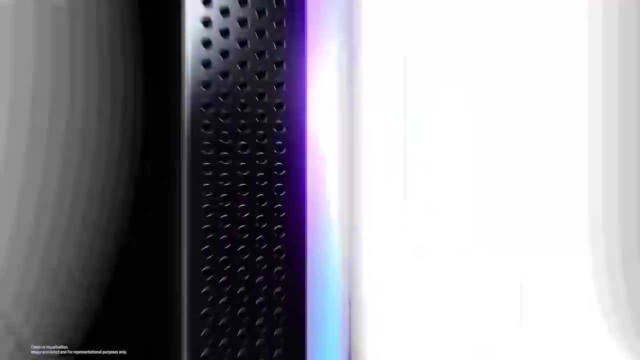 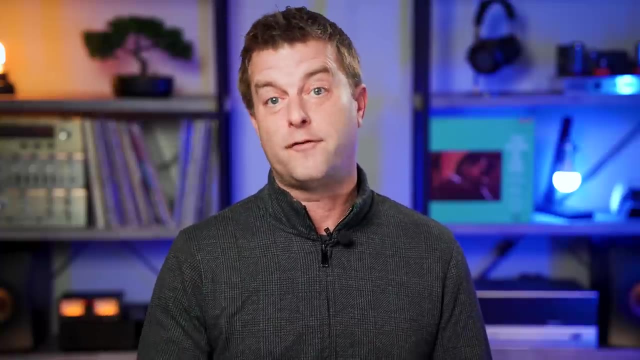 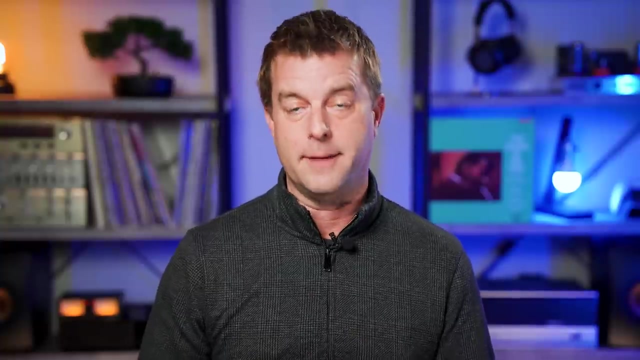 non-QLED LCD TVs for high dynamic range or HDR, And there's a ton of HDR content out there now coming from streaming services and 4K Blu-rays. We're even seeing some HDR content coming through some cable and satellite channels and it is gorgeous stuff to look at. Anyway, QLED TVs are 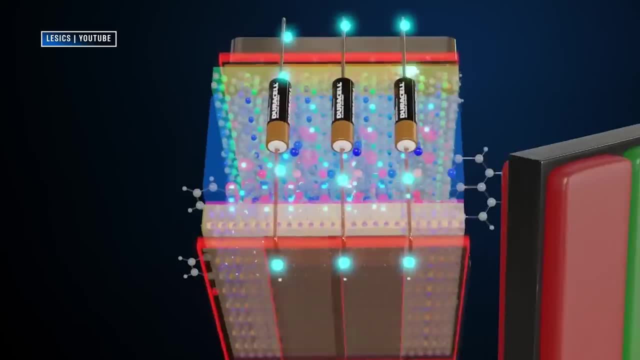 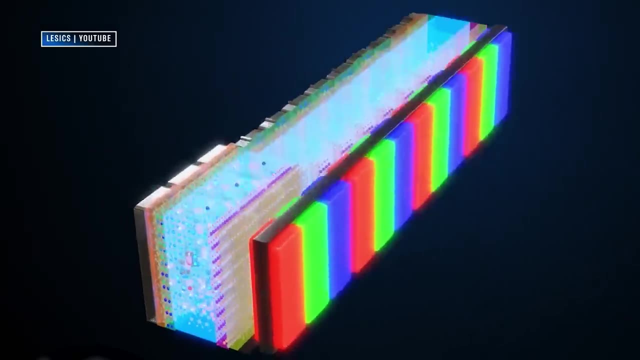 the best of the LCD TV camp. OLED TVs are a different kind of LCD TV and they're better of technology where each pixel makes its own light, no backlight required, And thus they have perfect black levels, which is the basis for amazing contrast. Now, it used to be that OLED. 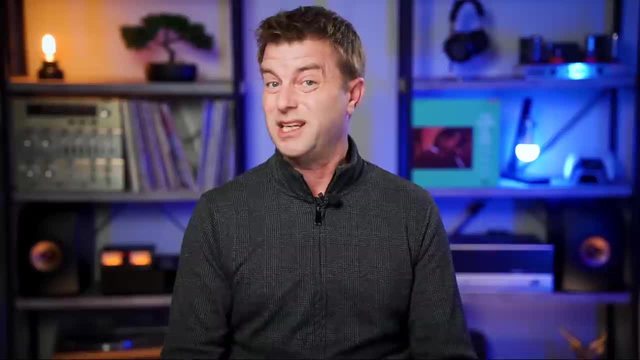 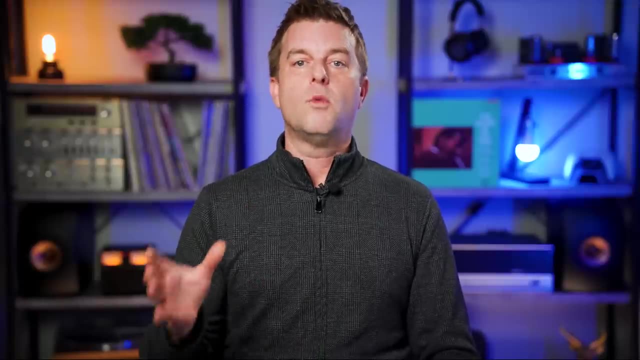 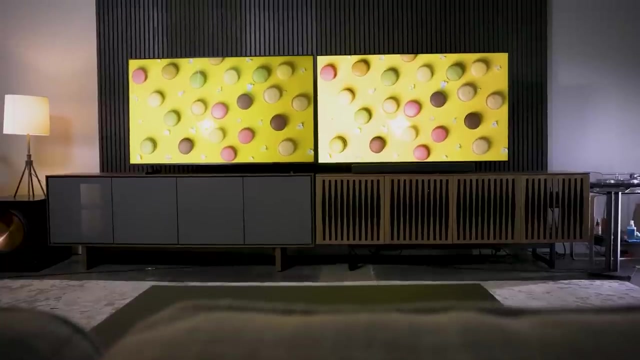 TVs couldn't get quite as bright as LCD TVs, but now they punch right up there in terms of brightness- Enough brightness for most folks in most situations. So we'll talk more about whether you might want an OLED or a QLED as we go down this list. Okay, let's start with the more. 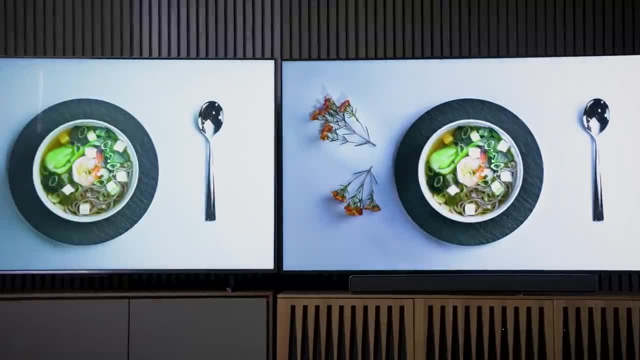 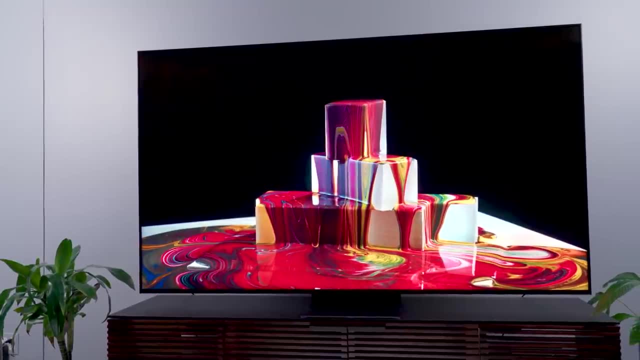 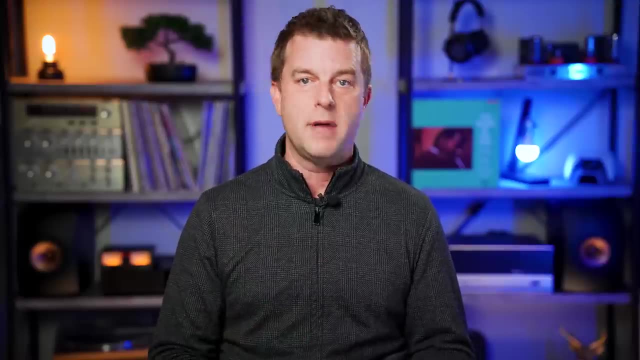 affordable, best QLED TVs and work our way up from there. It's a toss-up, really, between two TVs: the Hisense U8K and the TCL QM8. So let's just talk about those two together. at the same time, These two TVs are very similar in that they offer tremendous performance for the price. 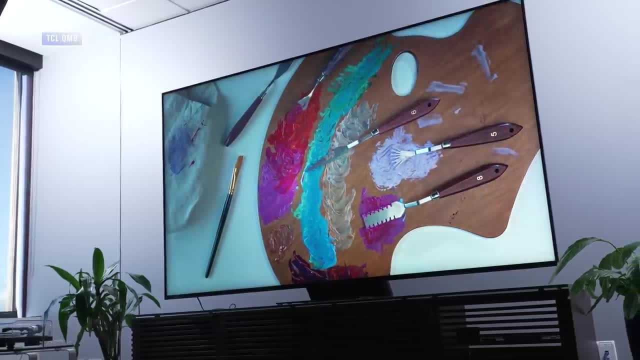 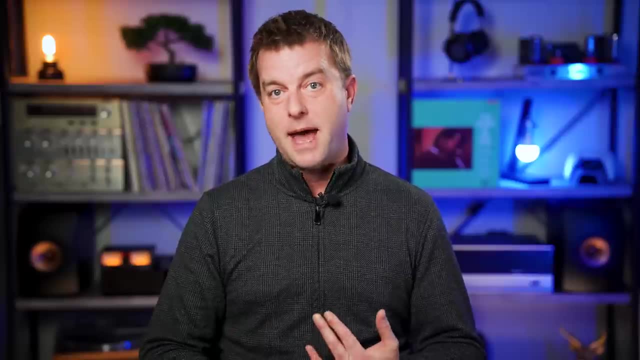 If you're looking to get the best picture quality you can for your money, these are the two TVs you should be looking at. Both of them offer class-leading brightness, excellent backlight control. so blacks are black and bright highlights have a lot of punch, and both offer. 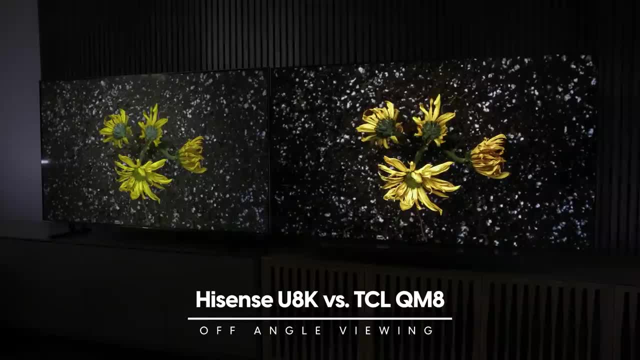 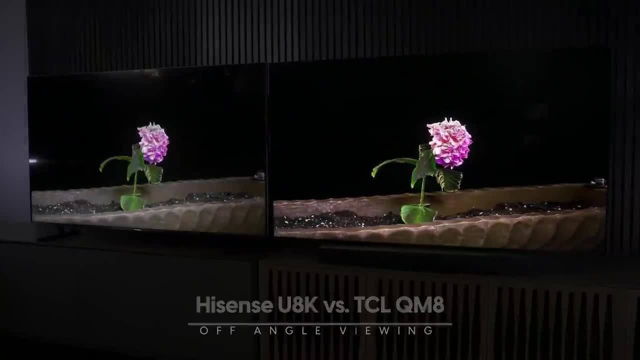 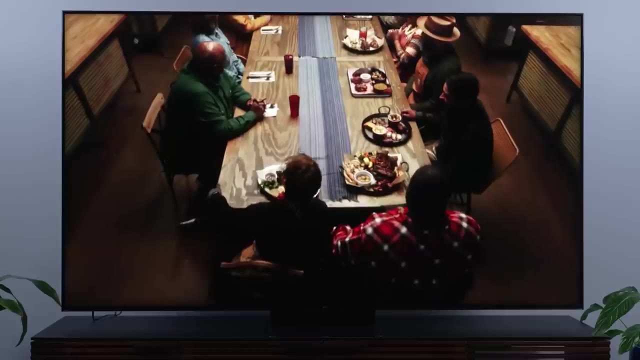 pretty accurate picture quality if you select the correct picture mode. These TVs are so close in performance that it was a tough call deciding between the two when I compared them. So if you're leaning toward one of these two TVs, I'd suggest checking out my comparison link below. Ultimately, 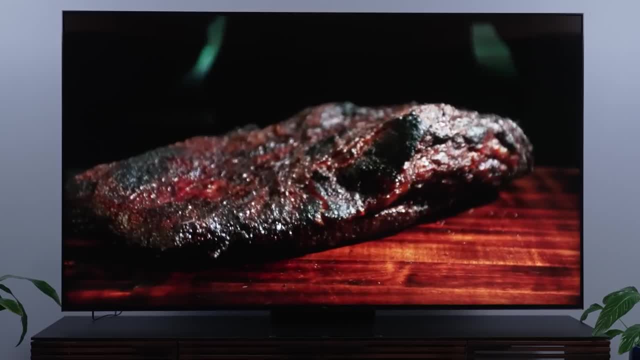 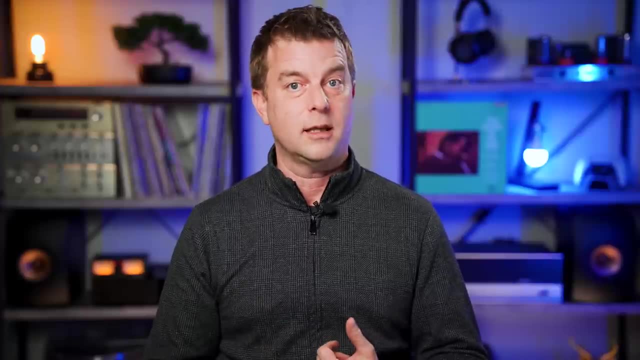 I ended up deciding that I'd probably lean toward the TCL QM8 personally, but not by much. The Hisense U8K is actually easier to adjust if you want to have the TV calibrated, which I understand is not something most folks are likely to do. but when searching for meaningful differences, 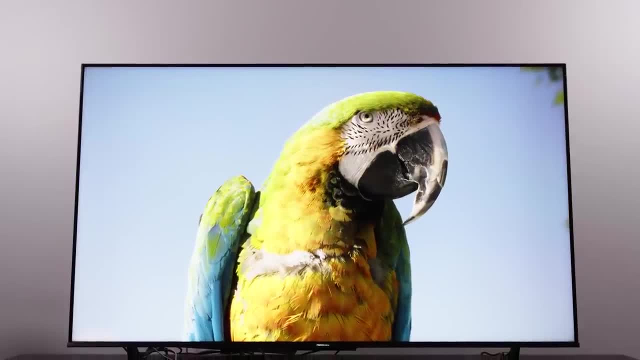 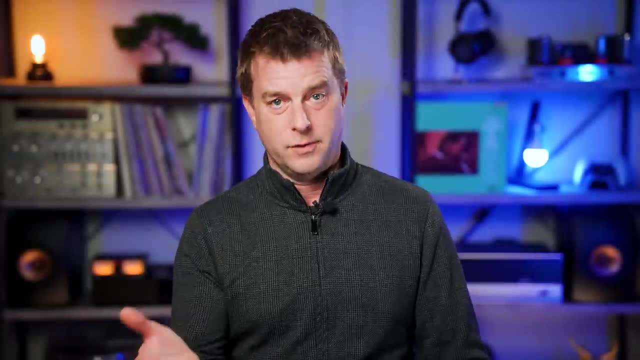 we have to drill down to that level. Also, the Hisense U8K has slightly better onboard sound quality, so if you're not going to use a soundbar or any other audio system, there's another reason to lean toward the U8K. Otherwise, I'm confident that most folks are going to be thrilled with. 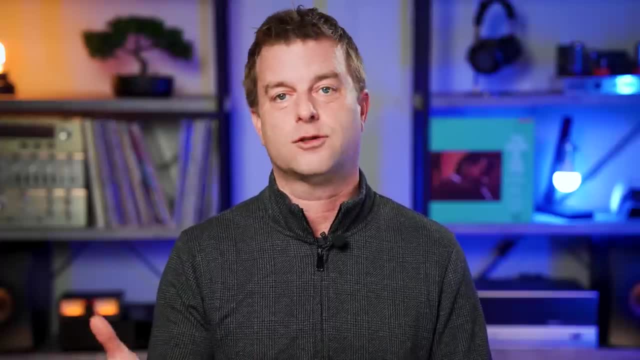 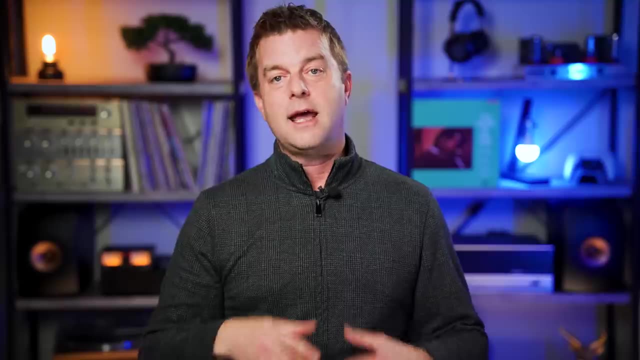 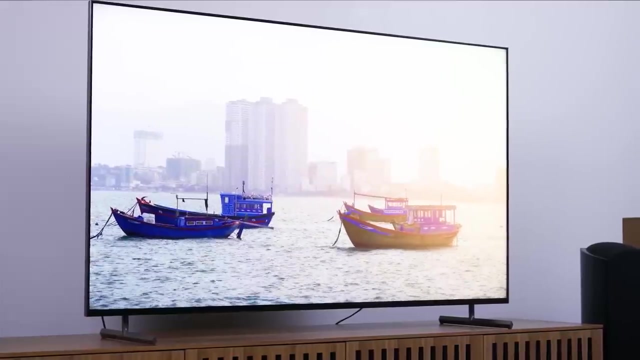 either one of these TVs. They really are just the easiest, and I can't wait to see what other recommendations I can make this year. Following closely on their heels is the Sony X90L. Now, depending on how deeply discounted TVs are when you're shopping, the Sony X90L may or may not be a little more expensive than the TCL QM8 or the. 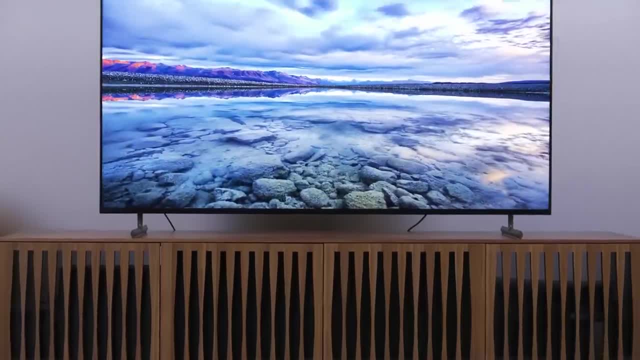 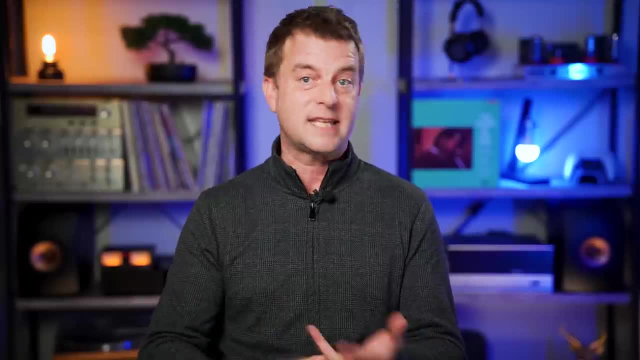 Hisense U8K. What I like about the Sony X90L is that it has better picture processing than the TCL or Hisense, And what that really means for you is that cable, satellite and other lower quality streaming devices are much more efficient than the TCL or Hisense, And that's because they're 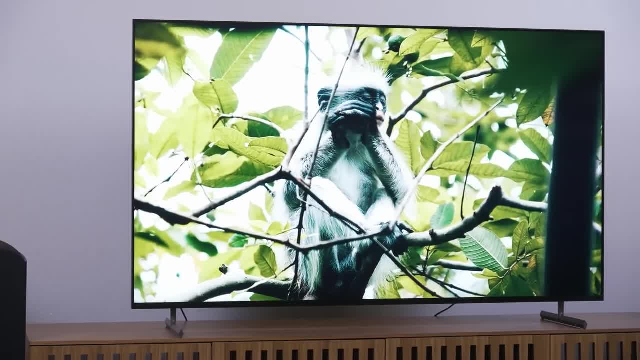 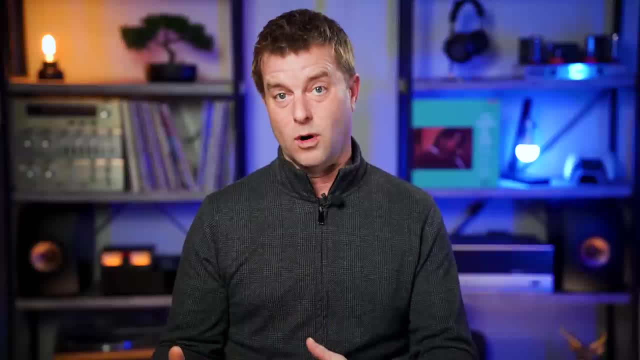 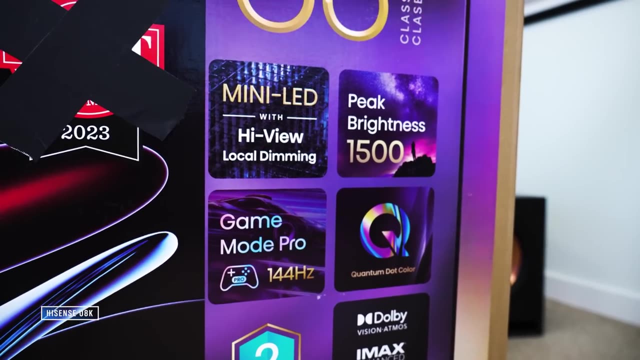 a little bit more expensive than the TCL or Hisense. You may pay a little more, but the Sony does make lower quality streaming content look better. Now the specs on the Sony may not look as impressive as those for the TCL and Hisense. 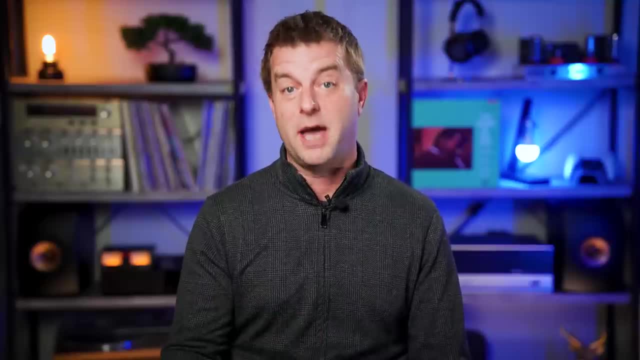 but in reality the picture is just as good, if not better, in most instances. I helped a close friend's family choose a TV recently. They wanted a 65-inch under $1,000 TV, but they didn't want it to look as good as the X90L. 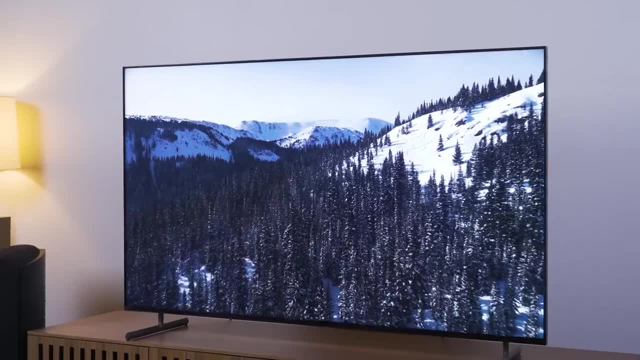 I was able to get a $1,000 TV for the X90L, and the X90L was my top recommendation. They got it and they are thrilled. Of course, they were also upgrading from a 14-year-old TV. 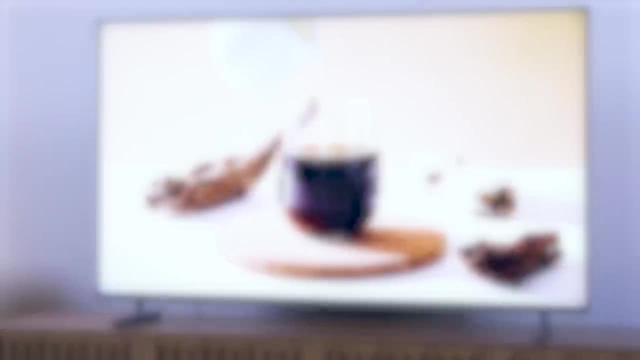 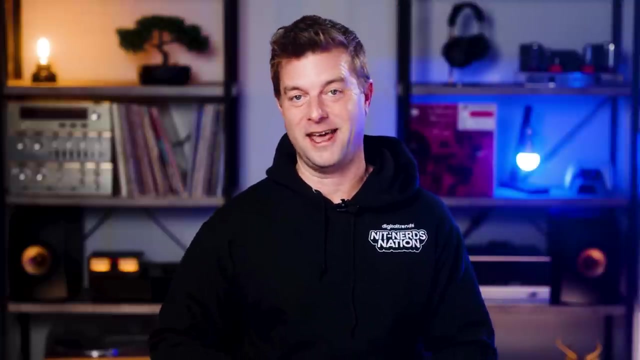 so it's a massive upgrade. Anyway, Sony X90L, my top pick for a 65-inch TV under $1,000.. Portable power stations are all the rage now, and I get it. Who doesn't love being able to power? 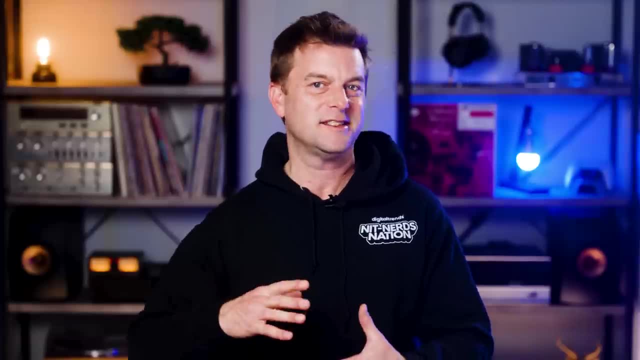 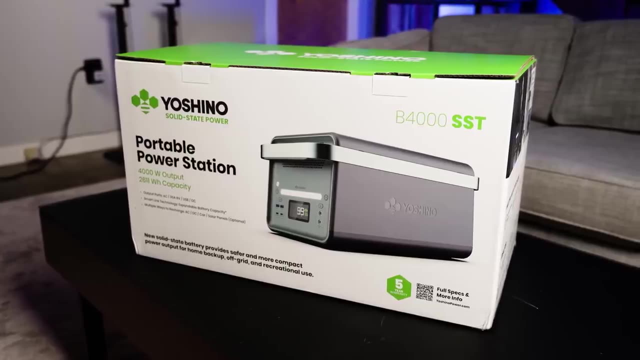 whatever you want, wherever you go. But now that the newness and novelty of portable power is starting to dwindle, folks are understanding that the X90L is a great option for the X90L, They are understandably demanding better. That's where the Yoshino B4000 SST comes in. 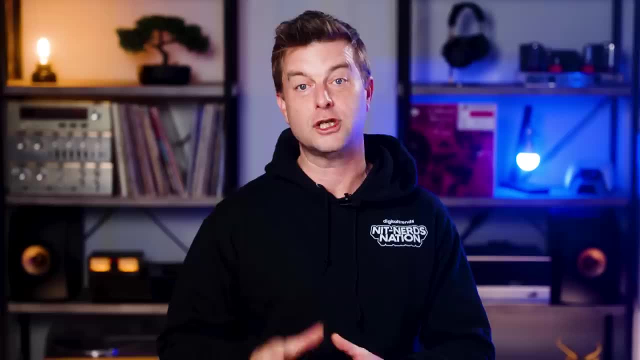 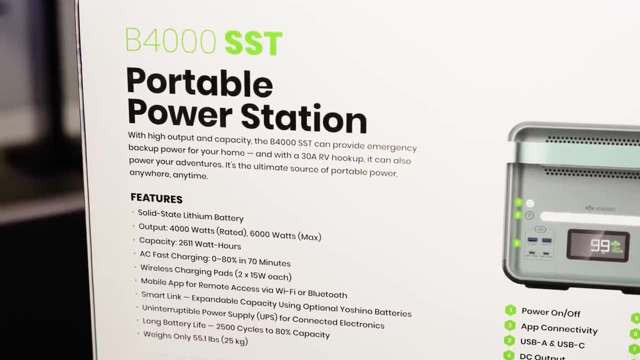 Those three letters, SST. they're the key here. Yoshino's solid-state technology is what makes its power solutions so advanced. Yoshino's solid-state solutions are more reliable, better for the environment and more practical than conventional lithium iron cells And with 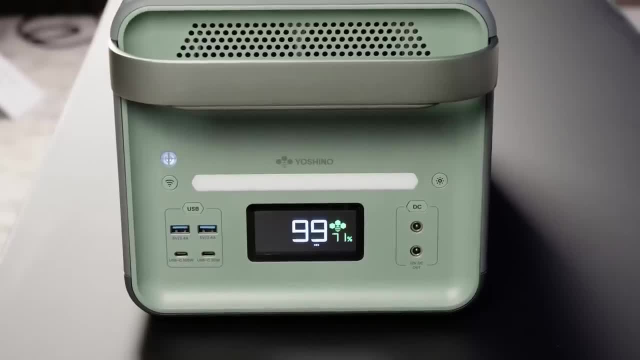 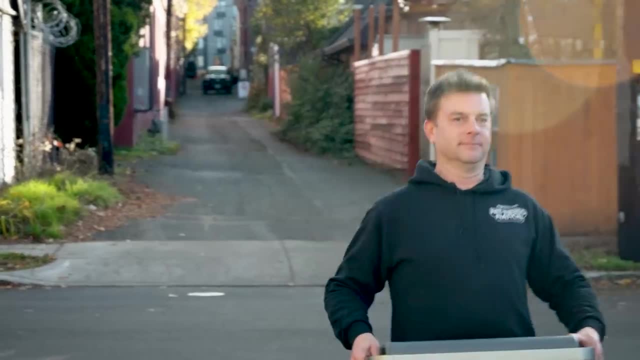 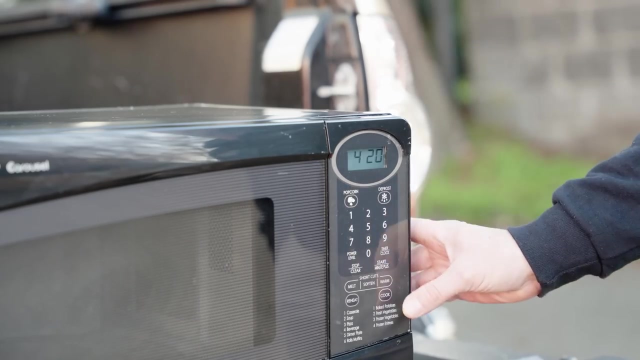 its light, compact, ergonomic design and soft-touch aluminum handles, the Yoshino B4000 SST is actually easily portable. The possibility doesn't come at the cost of real power. The B4000 SST packs the punch of much larger, heavier portable power stations. 4,000 watts of power is on tap here with a 2.6 kilowatt hour. 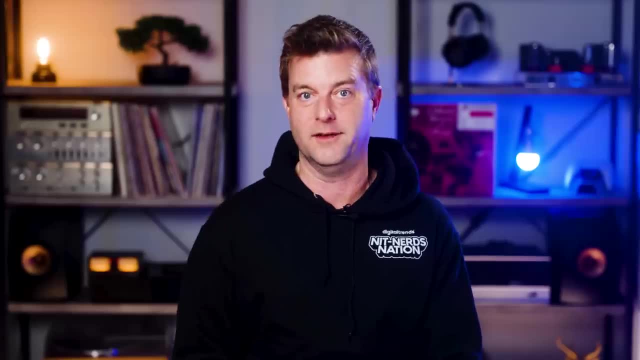 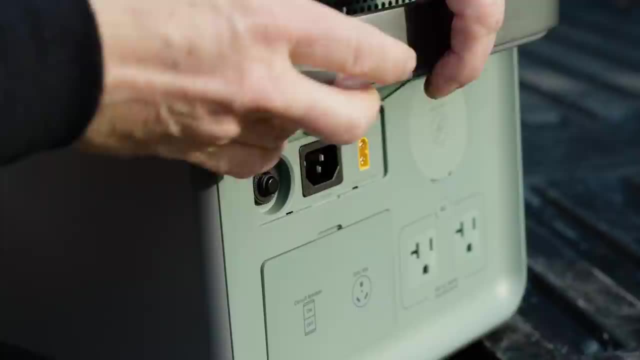 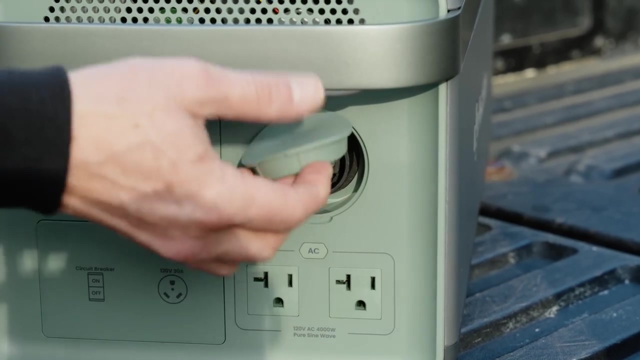 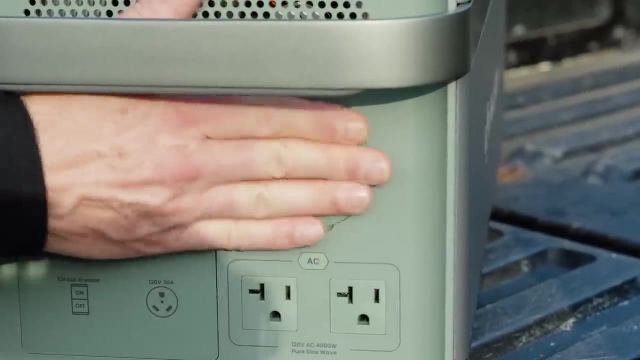 capacity in this. Can you believe that? Believe it And look. you've got all the connections you need and expect: USB-C, USB-A, DC power ports, AC power ports, wireless charging pads. it's all here. You can plug your RV in directly, Leave your adapter dongles at home And, as an avid RVer, 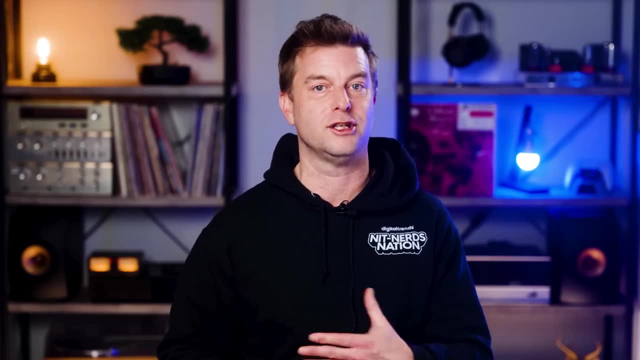 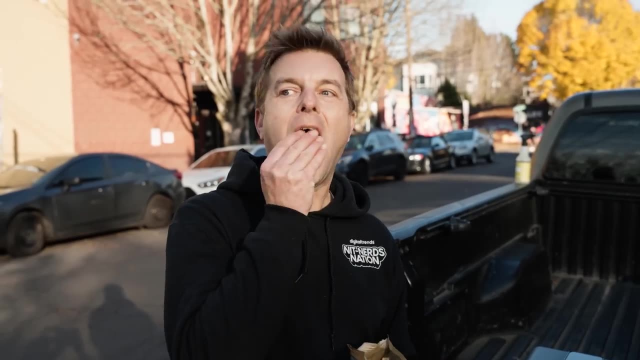 I love. that Doesn't matter whether you're at home, a campsite or a job site. the Yoshino B4000 SST is out of sight, Literally. It's so compact you can tuck it away. It's like invisible power. But why? 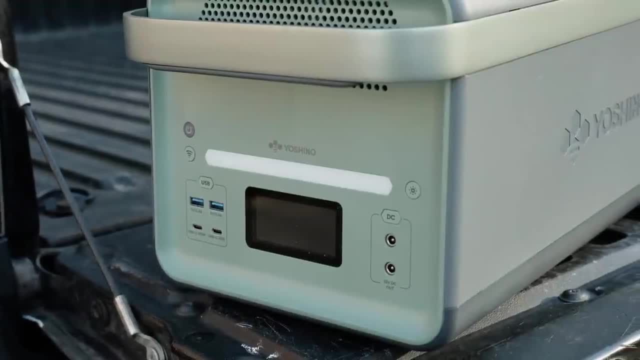 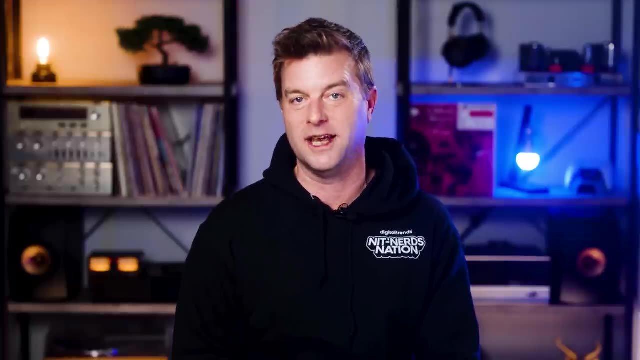 hide it. This thing looks so cool. Best of all, we have a huge deal for you on the B4000 SST: $800 off for the holidays. Just click the link down in the description for instant savings. Thanks again to Yoshino for sponsoring this portion of our video. 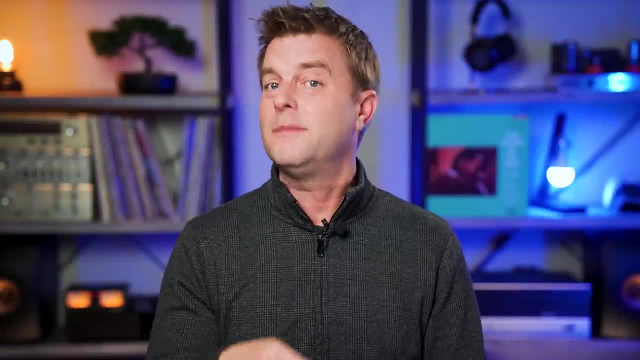 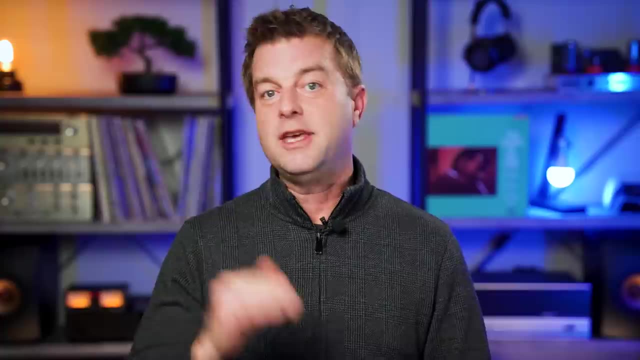 Now let's step up to some more premium TVs. This is where you'll start paying a bit more, but you'll also get some more refinements to the picture quality and some added features. These next two TVs are what I think are the best QLED TVs for this year. The first I'll mention is the 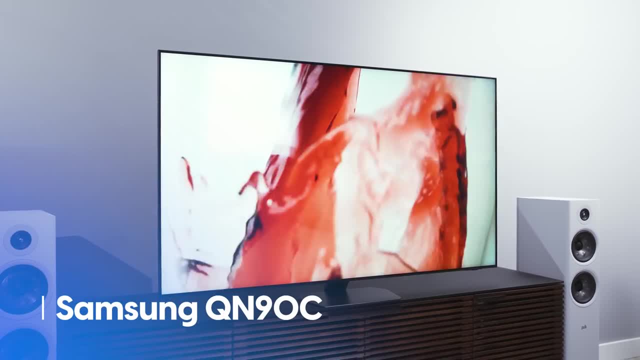 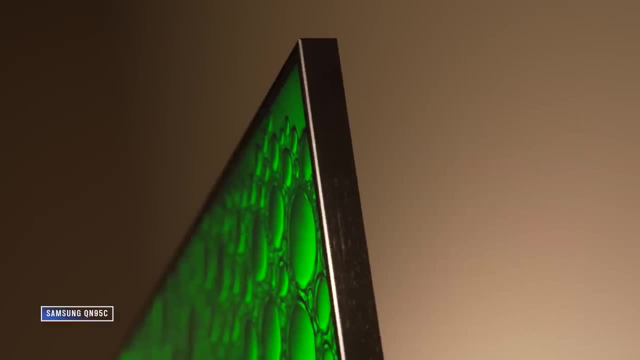 Samsung QN90C. Now, some of you out there may be wondering why I'm not talking about the QN95C, which is one step above this TV, or why I'm not recommending one of Samsung's 8K TVs. Well, I'm not going to recommend one of. 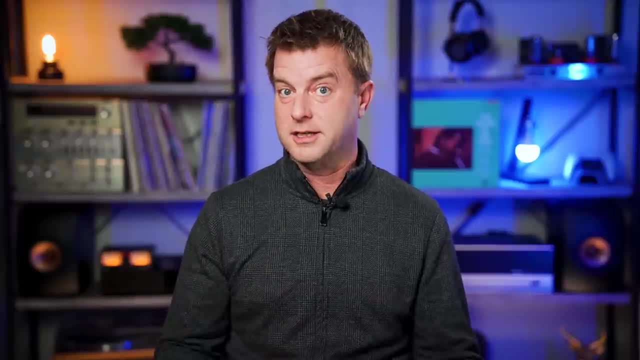 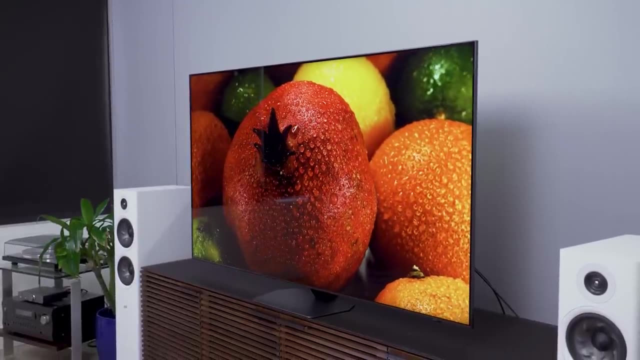 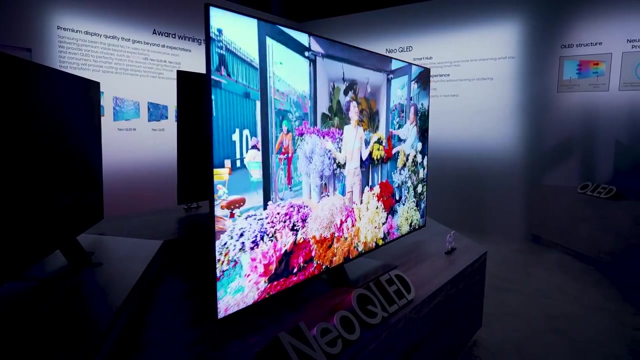 Samsung's 8K TVs because, while they are definitely stunning, I don't feel they offer enough benefit over Samsung's best 4K TVs to justify the bump in price. You may notice that none of the TVs I'm recommending are 8K TVs, and that's because I just don't feel that they serve many people that well. 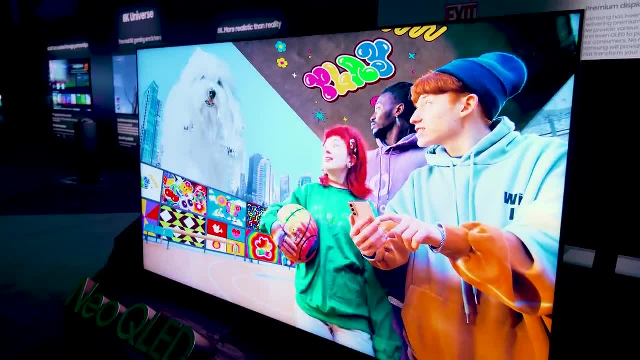 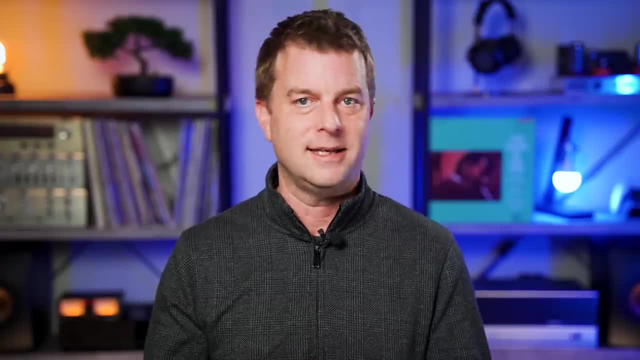 If you've got tons of money to burn, sure, get an 8K TV. they have the best tech in them and you won't be disappointed with any of them. but there's really no deliberating among 8K TVs because there are so few of them. It's 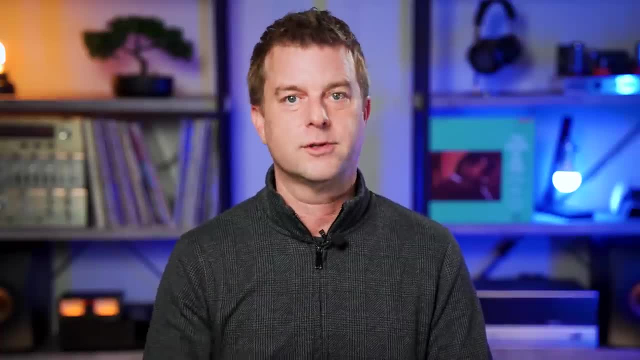 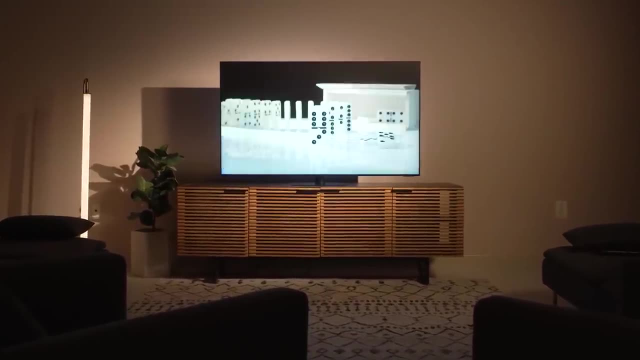 harder to choose among the best 4K TVs, so I'm sticking to those. As for the QN95C, why am I not recommending that one? Well, I don't know what the deal is with that model, honestly, but it is not easily buyable at retail anymore. I think you. 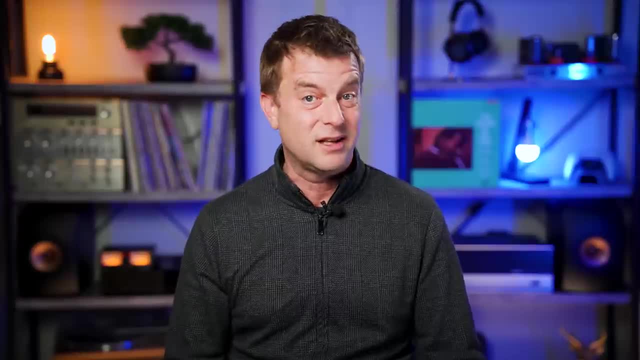 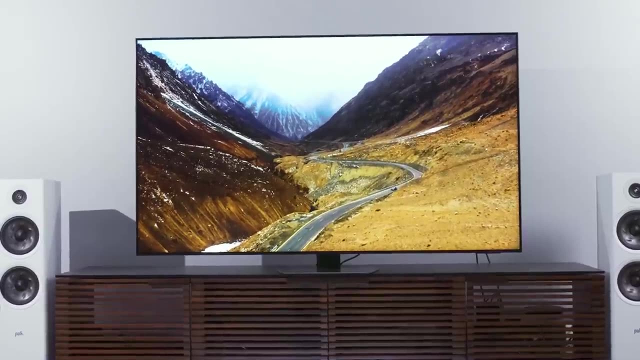 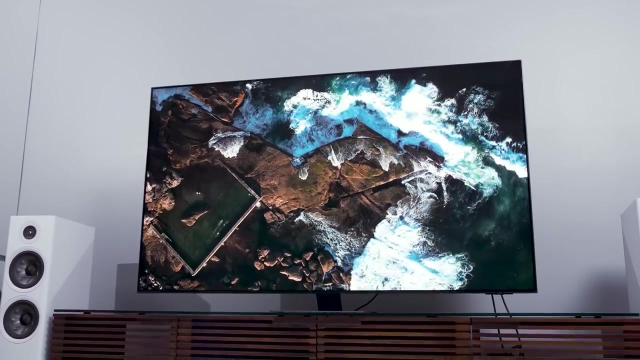 can get it from custom installers and from some oddball retailers, but it's not in stock anywhere yet, which is why I'm going to stick with the QN90C Plus. the QN90C is just a tremendous TV overall: Super high brightness, excellent backlight control, vivid color, solid picture processing. 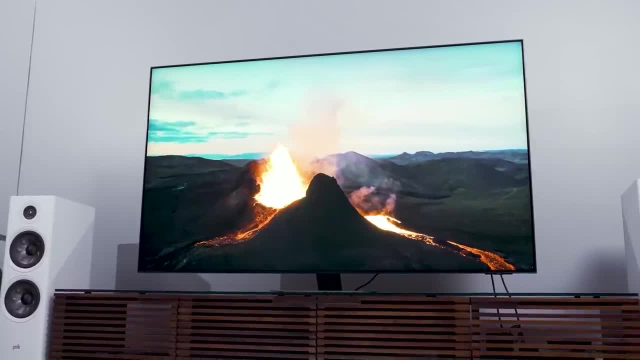 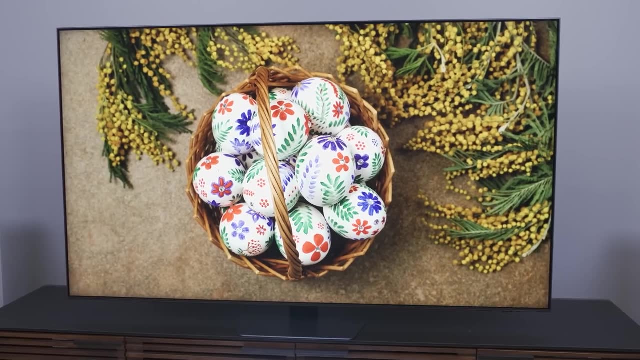 but I'd say the QN90C's real ace in the hole is its off-angle viewing and its anti-glare capabilities. This TV makes just about any seat in the house the best seat in the house, so if that sounds like something that you need, the QN90C might be the best QLED choice for you. 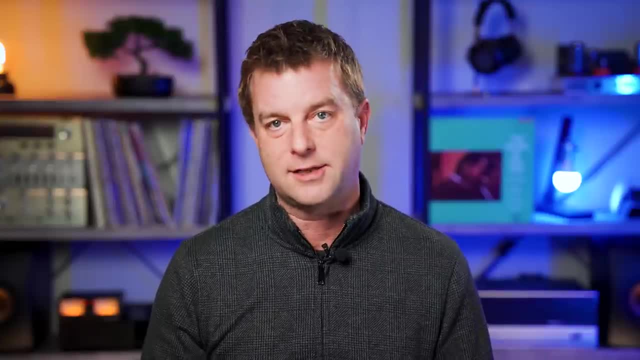 It's got a lot of features, but it's also got a lot of features that you don't want to miss out on. It's got the best off-angle viewing of any of the QLED TVs on this list and it's second only to OLED. 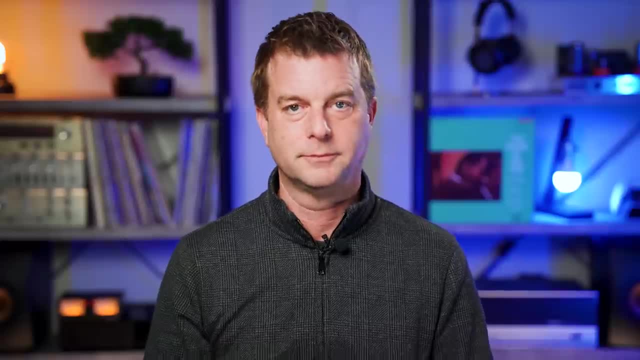 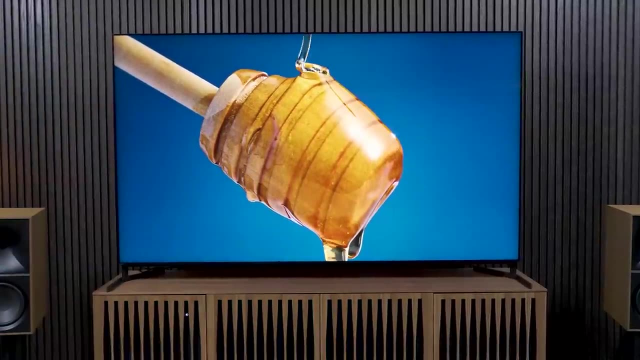 TVs in off-angle viewing, which I'm going to talk about some later. Up next, the Sony X95L. It's my choice for the best QLED TV of the year and you'll pay handsomely for it. but what sets the X95L apart? 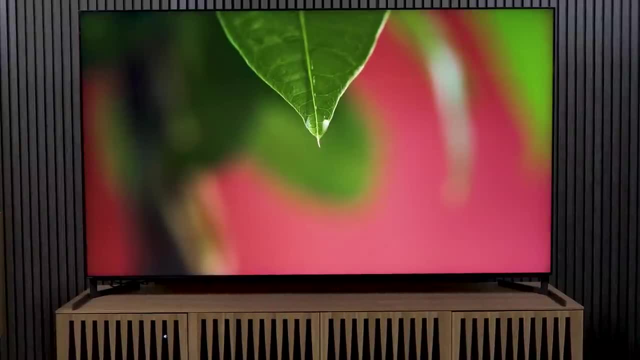 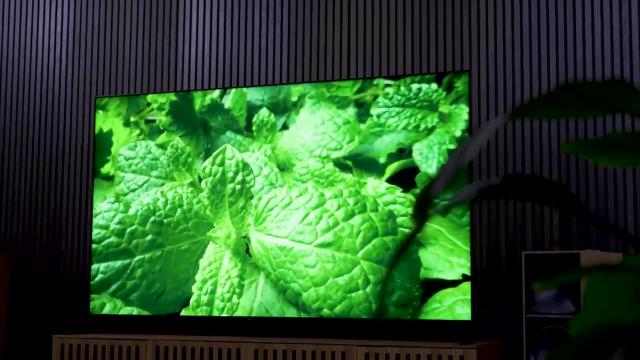 from the rest is what sets any Sony TV apart from its competition, and that is the picture processing. It's just an exceptionally clean-looking TV with punchy brightness, excellent contrast, the best upscaling, the best improvement to low bitrate content like cable. 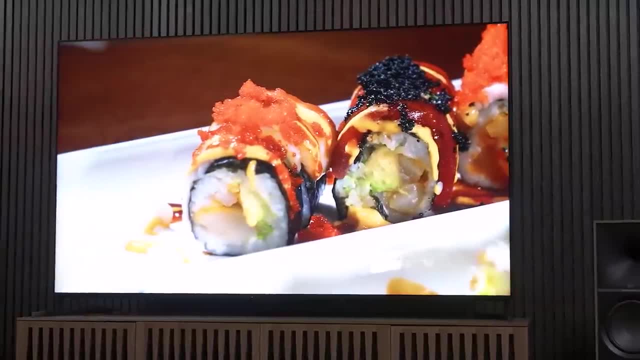 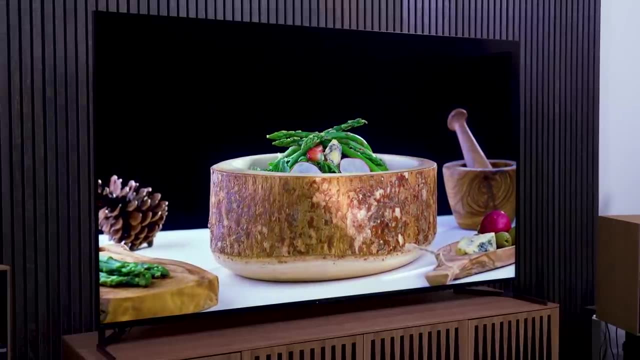 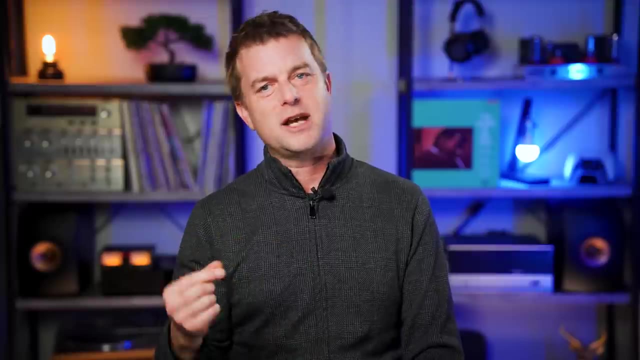 satellite and live streaming TV services and the best cinematic motion. If you're real picky about picture quality and accuracy and willing to pay the premium, the Sony X95L delivers Okay. one last QLED TV before we move on to OLED, and this is kind of a special one that 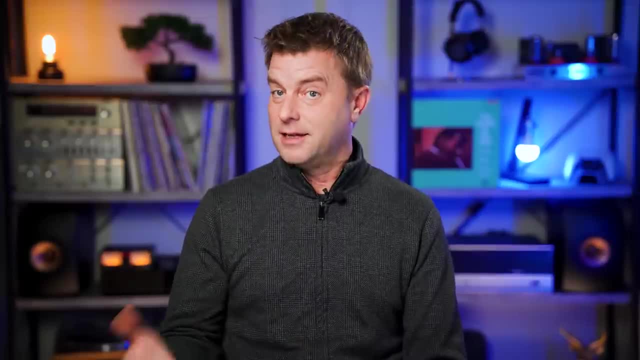 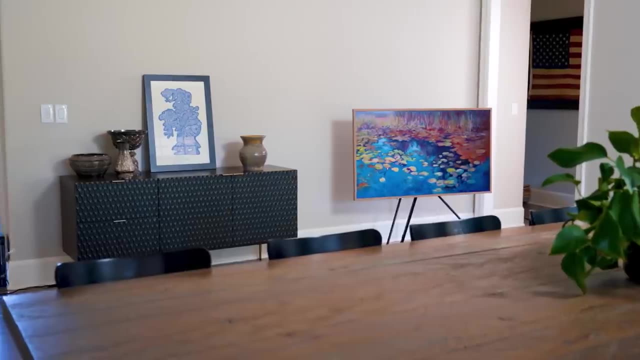 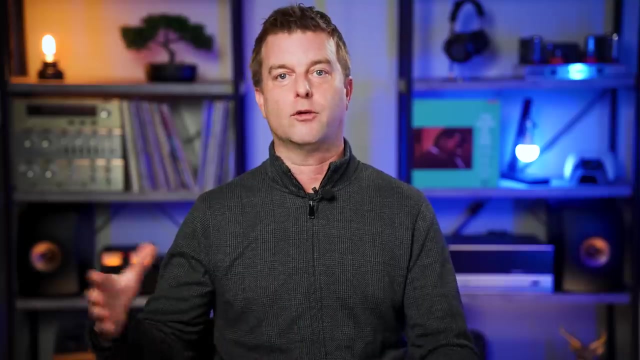 resides outside the list of conventional TVs. It's a novelty, but it is not A gimmick. I'm talking about Samsung's The Frame TV. Folks, if you want your TV to be more than a TV, more like a work of art when you're not watching it, rather than just being a big black rectangle. 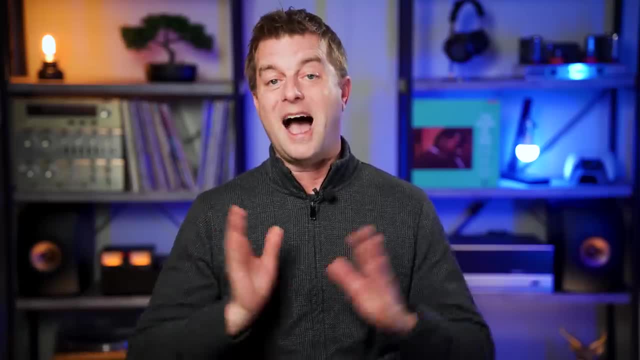 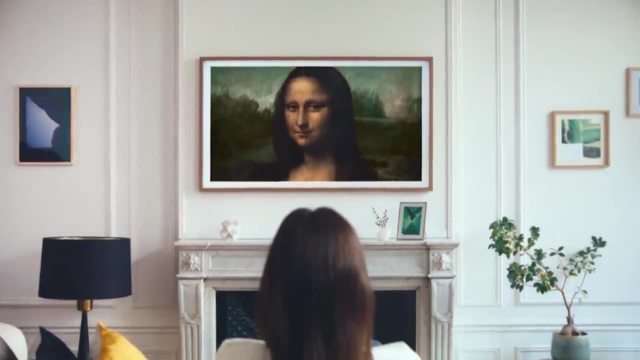 in its off-time, then The Frame is for you. I cannot overstate how realistic art looks when this TV is displaying it. The Frame TV looks like art on a canvas, and that's thanks to its special matte finish, Also as a bonus. it's really good. 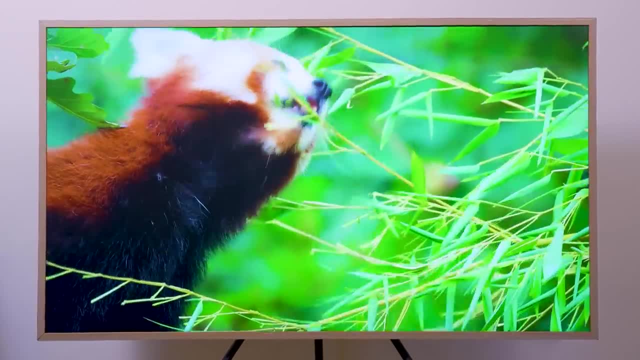 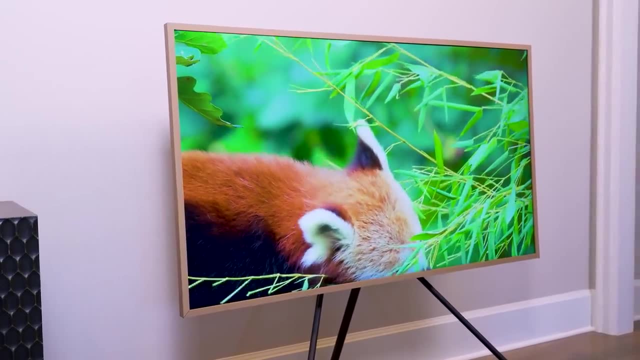 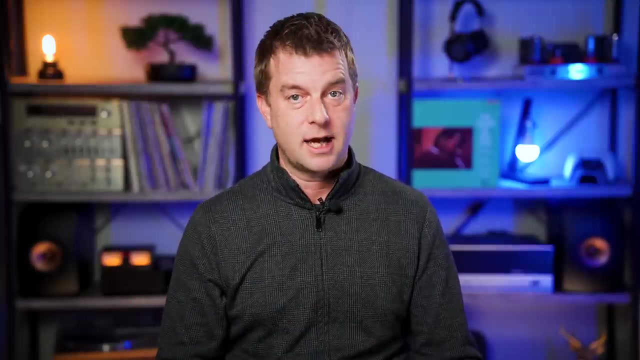 bucking glare. so if you have a bright room with lots of windows, The Frame does a great job handling reflections so that you see the content, not your reflection. It's a solid- I mean remarkable- HDR TV that doubles as a work of art, and it comes in a wide range of sizes. 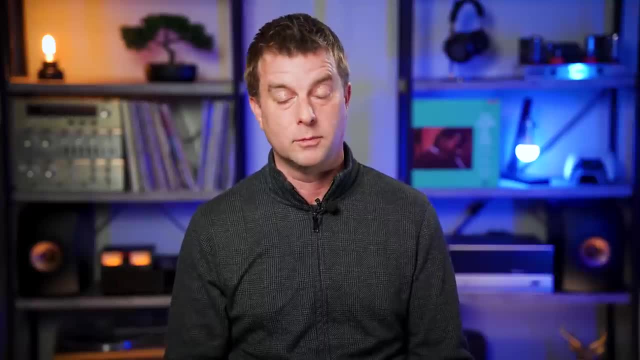 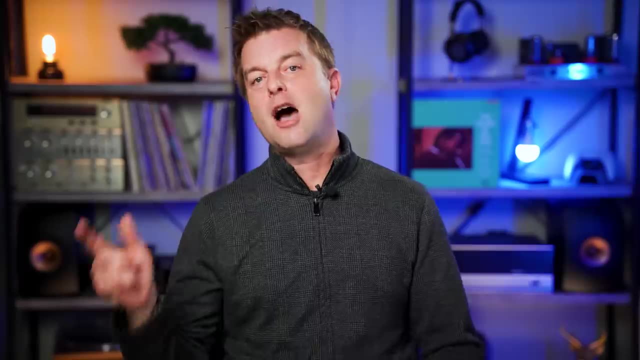 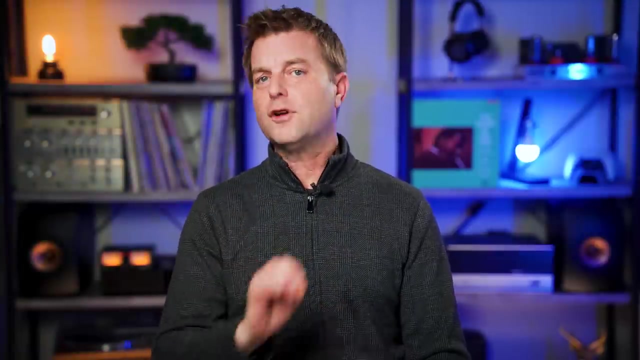 I've even seen some folks use more than one in a room. I cannot say enough good things about The Frame TV as a lifestyle TV choice Highly recommend. And now, my friends, we switch gears to the OLED TV options on our list. Before I start running down the model options, let me first 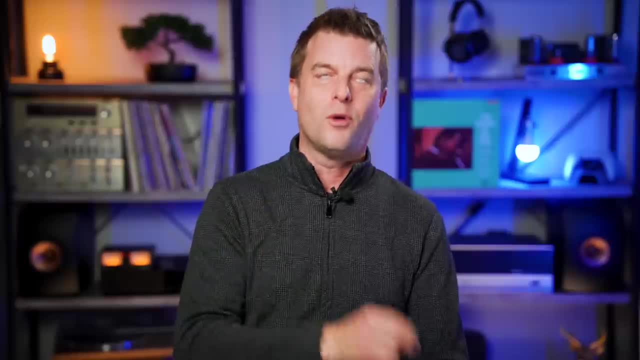 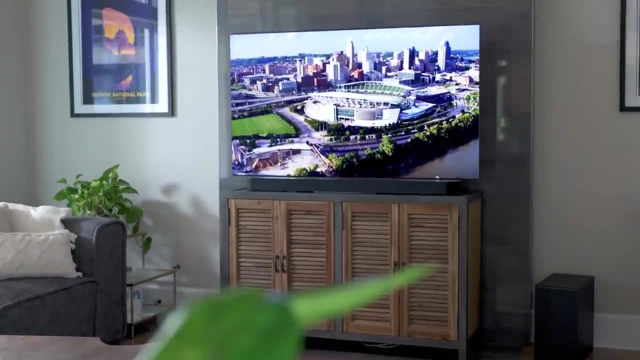 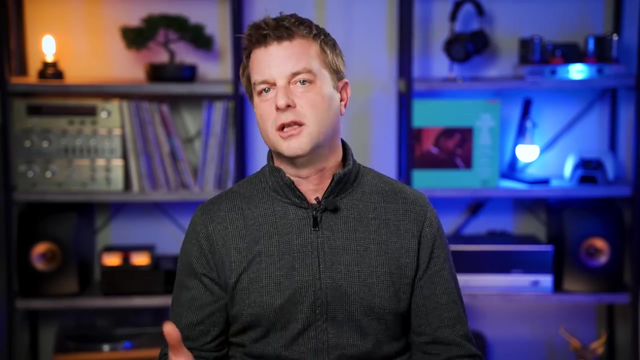 clarify who an OLED TV is good for and perhaps, more importantly, for whom an OLED TV is probably not a good choice. I say: get an OLED TV if you are really deliberate about liking to sit down and watch TV. Watching TV for you is a real occasion. You make watching sports a big deal. You make 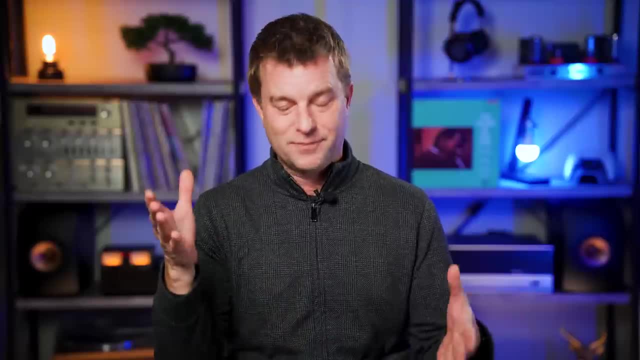 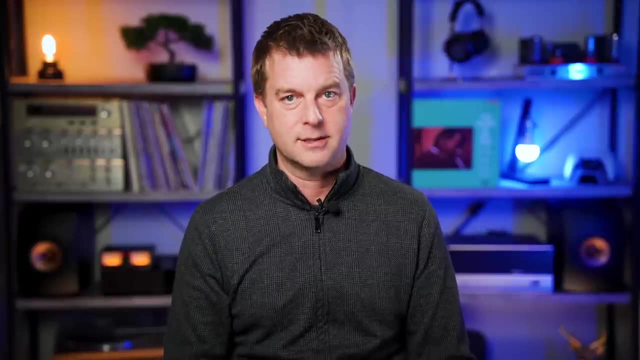 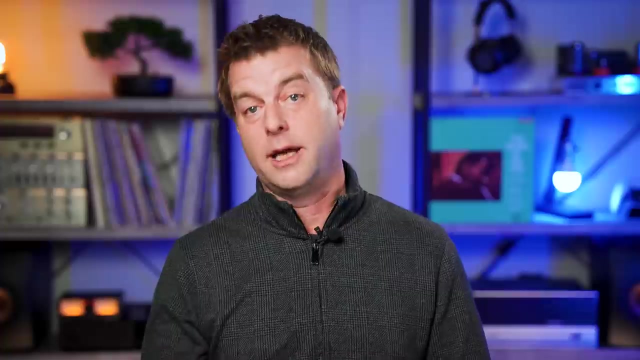 picture quality possible, and when you sit down to watch TV it's a real treat. Maybe you have a dedicated media room or a home theater. OLED is a great choice in those cases. OLED is probably not the right TV type for you if you turn on your TV in the morning and you let it run all day long. 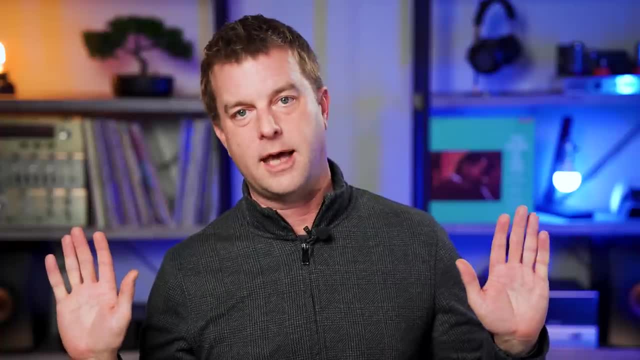 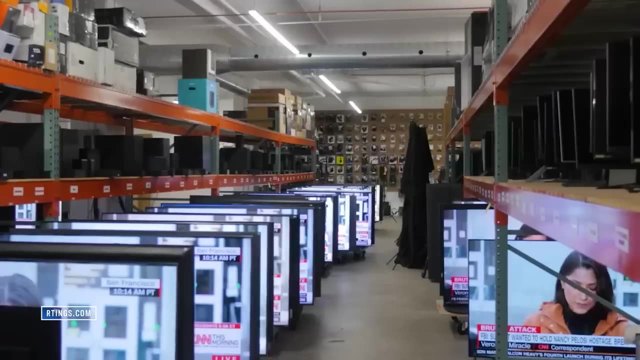 That's a popular thing to do and I make zero judgements about that, But because OLED TVs are susceptible to burn-in under high-intensity use conditions, someone who puts on ESPN or or any other channel with a Chiron- that's the info banner at the bottom of the screen. 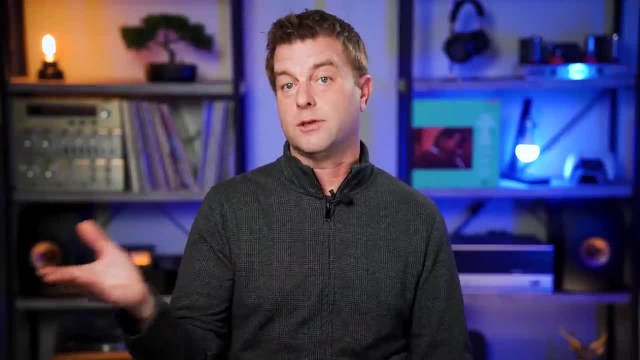 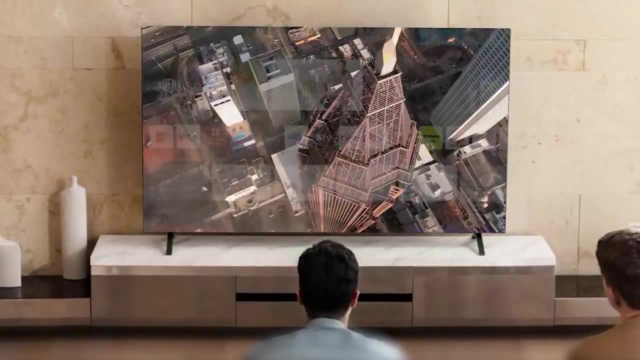 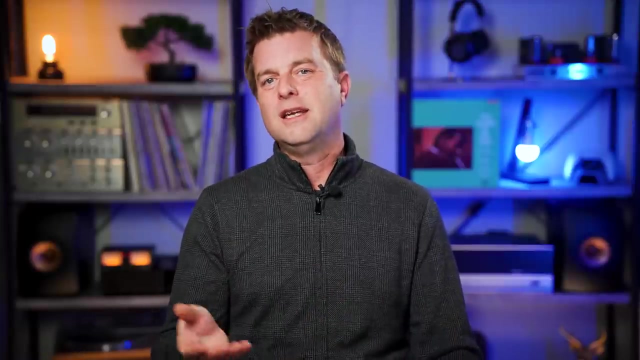 that's always on and leaves the TV on for 12 hours or more. there's just too much risk long-term of wearing out an OLED TV, even today, when OLED TVs have a lot of built-in measures that help prevent burn-in Plus, frankly, paying a premium for an OLED TV. 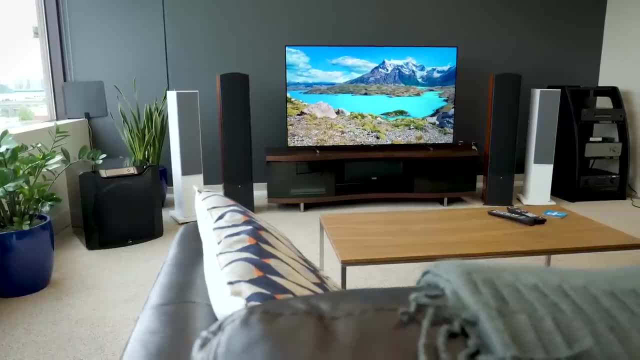 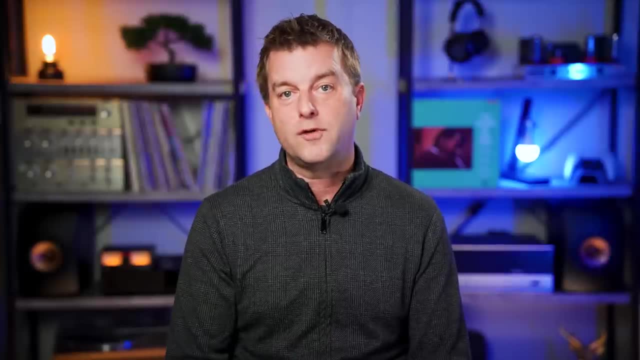 just seems like a waste if you aren't spending most of the time the TV is on sitting down and enjoying it. OLED TVs just aren't a great background TV and I know that's a popular type of use, so keep that in mind. 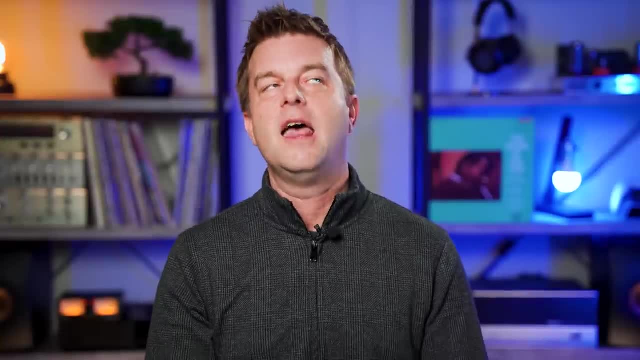 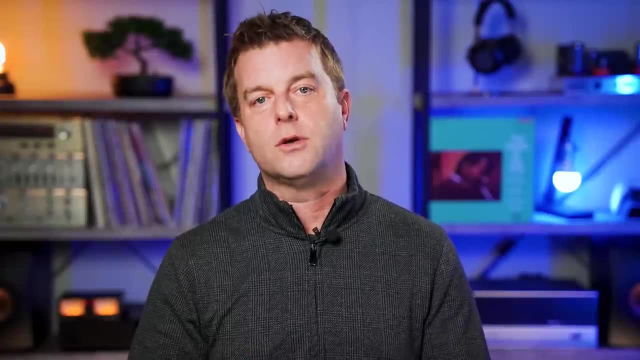 But if you do consider yourself a good match for an OLED TV, they are gorgeous, still the best picture quality you can get. So let's talk about the best OLEDs you can buy, and each of these is gonna have a step-down option too. 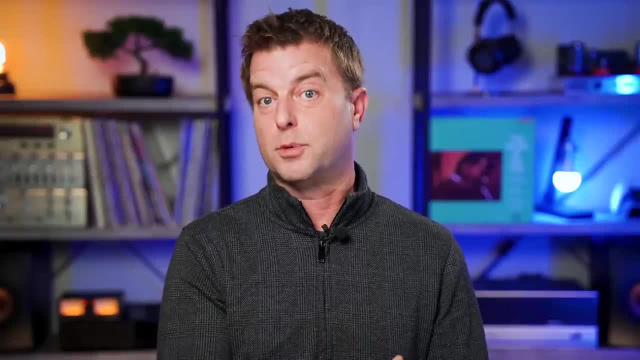 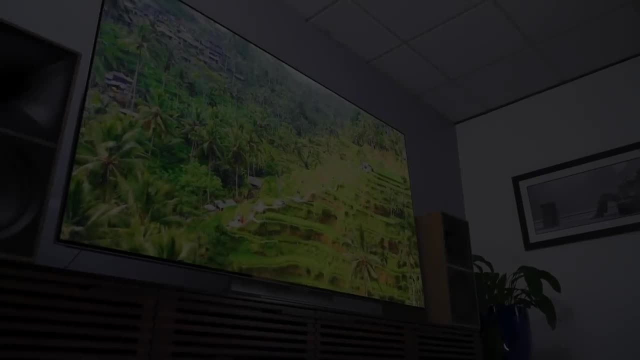 that will offer you like 90-something percent of the flagship's performance for less money. so you've got options. The first OLED TV we'll talk about is the LG G5. It's the G3 Gallery Series OLED. This OLED has, in my experience, 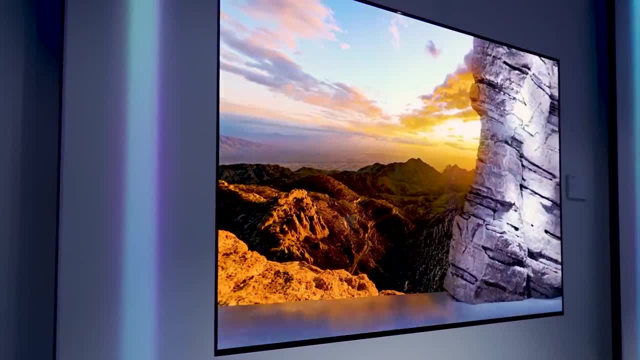 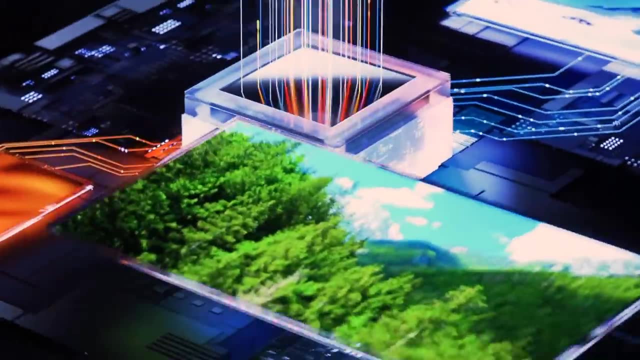 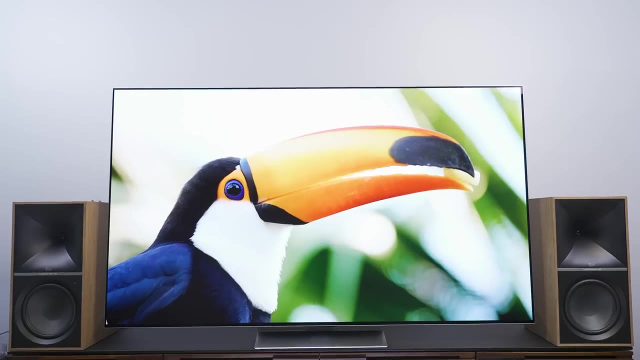 the highest perceived brightness of the OLEDs on my list. That's thanks to what LG calls MLA or Micro Lens Array technology, which is a super thin layer of tiny little lenses that focus light out to you, the viewer. The G3 is capable of stunning picture quality. 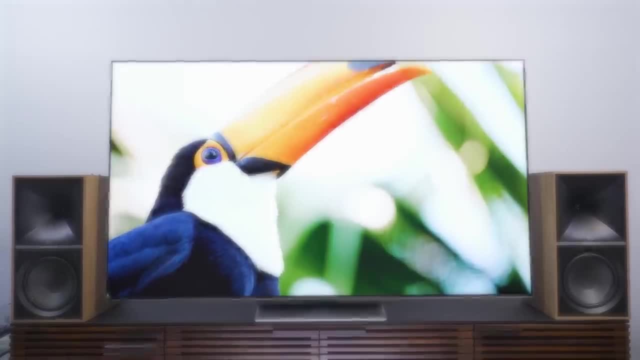 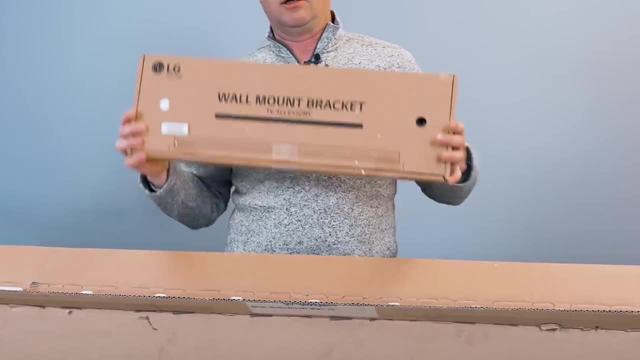 and it is loaded with features. The one catch with this TV is that it does not come with a tabletop stand. It's meant to be mounted on the wall, but the good news is that LG provides a no-gap wall mount right in the box. 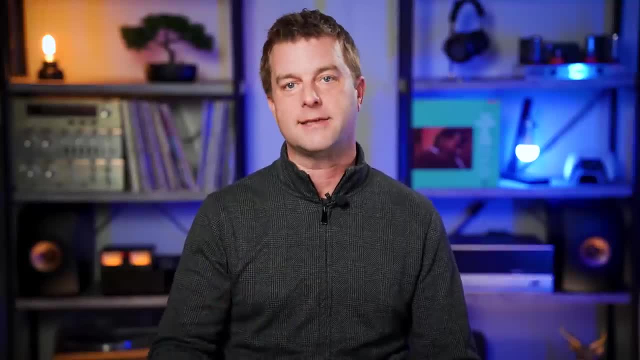 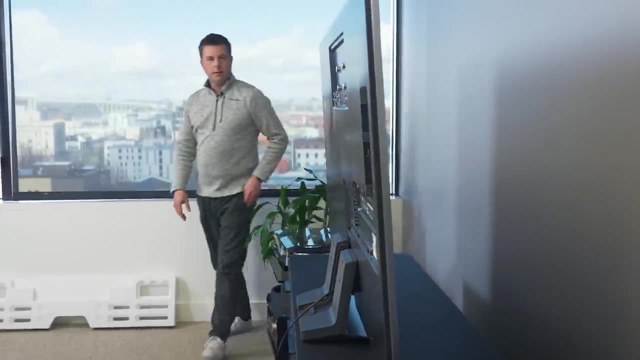 so that when you mount this TV, it's as flush against the wall as it can be, which yields a very sleek look. You can buy a tabletop stand for the TV. LG sells a rotating Lazy Susan-style stand, but I'm not a huge fan of it since it's kind of wobbly. 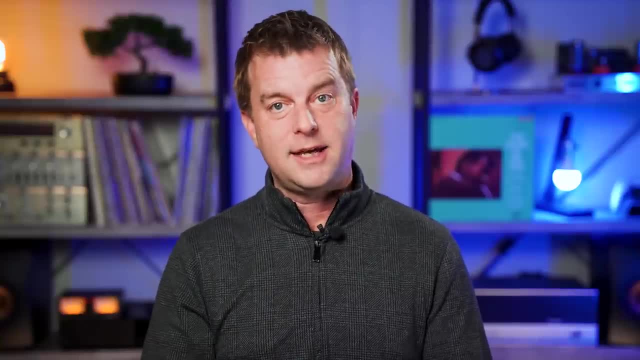 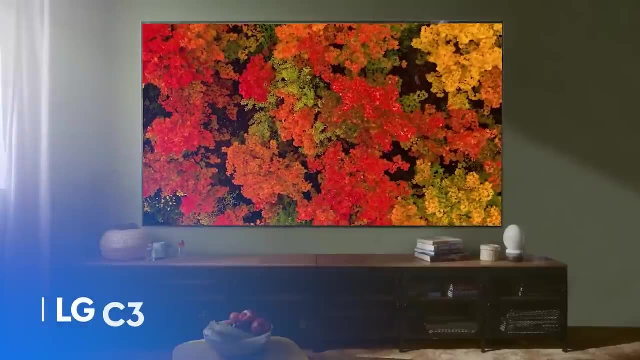 You can also buy third-party stands that screw into the back of the TV. but I mean, I just don't think they look all that great. This TV really is best wall-mounted, And if the G3 is a little rich for your blood. 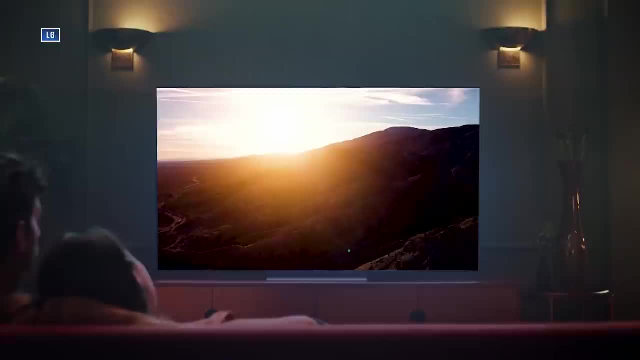 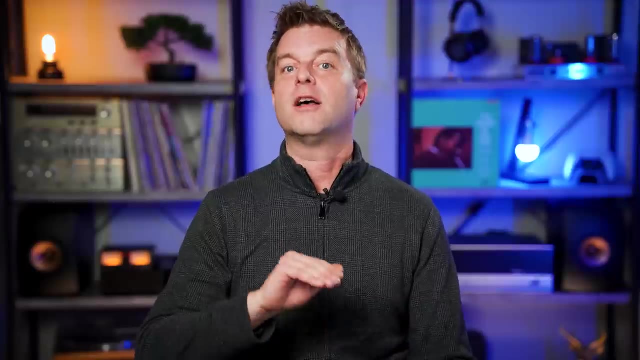 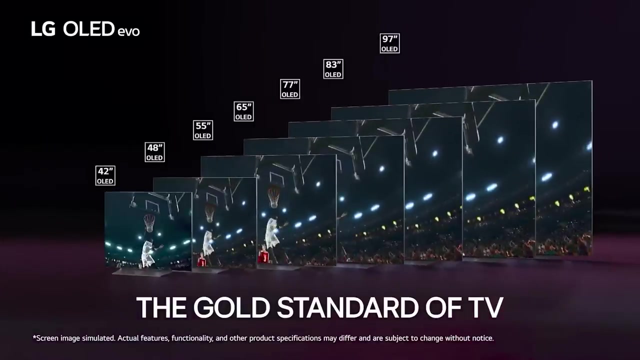 check out the step-down LG C3 OLED. It isn't quite as bright as the G3, but it is plenty bright for most folks and it comes with a stand and it costs significantly less. Oh, and one last thing: The LG G3 and C3 can both be had up to 83-inch screen sizes. 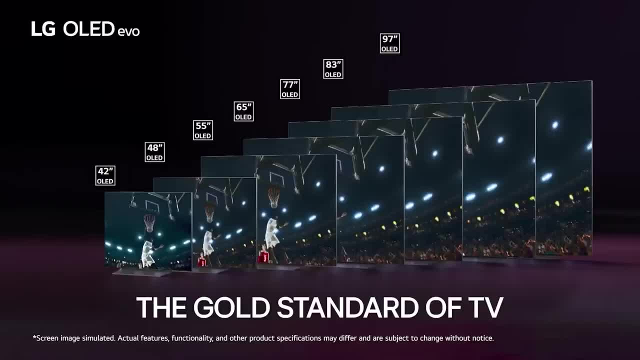 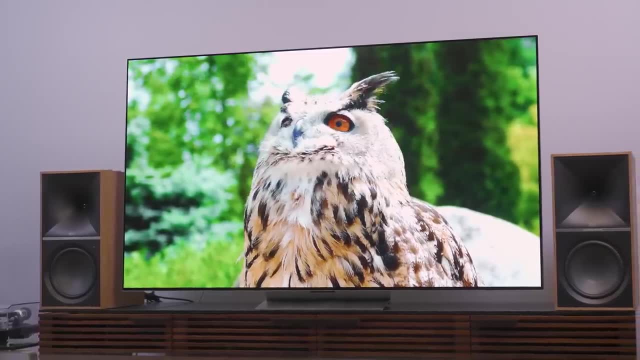 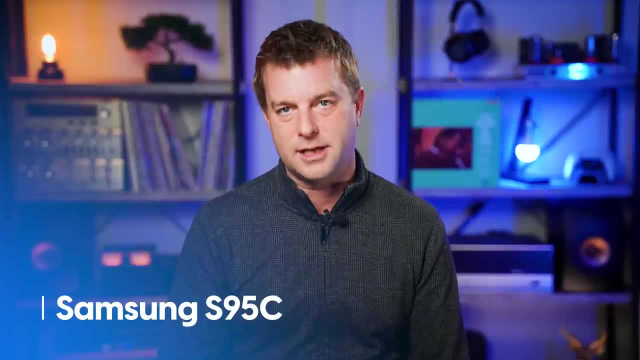 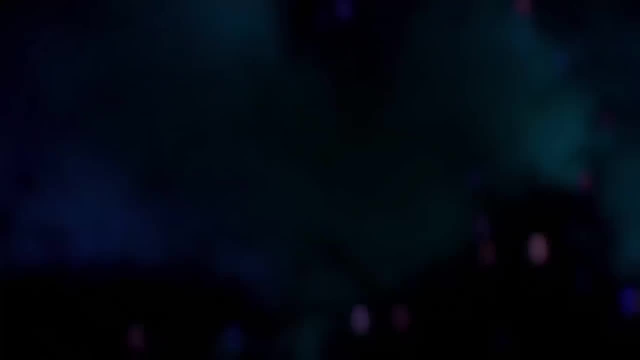 Next OLED TV on this list is the Samsung S95C OLED. This OLED TV uses a new Quantum Dot OLED panel, also known as QD OLED, and the trick up this TV sleeve is that it can emit very pure, high-brightness colors. 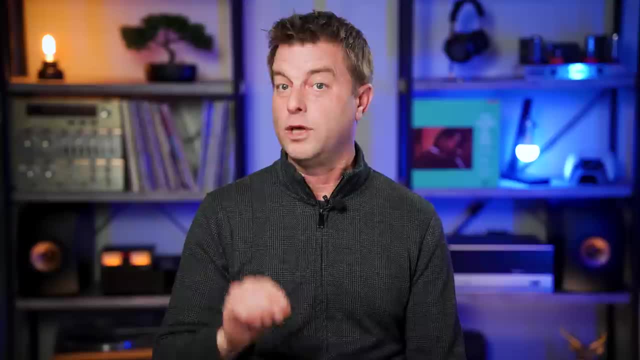 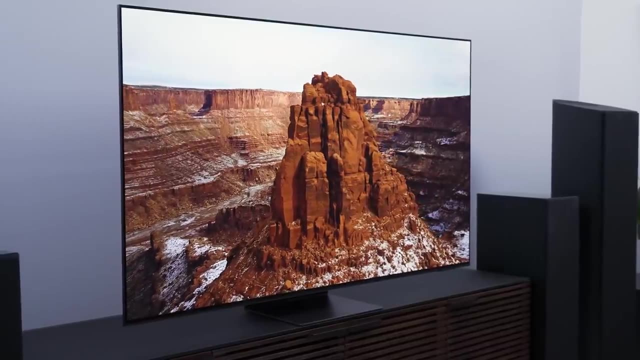 It's hard to describe what that experience is like, but when you see it you'll know what I'm talking about. And as a top-tier Samsung TV, this thing is loaded with bells and whistles, including some audio tech that works exclusively. 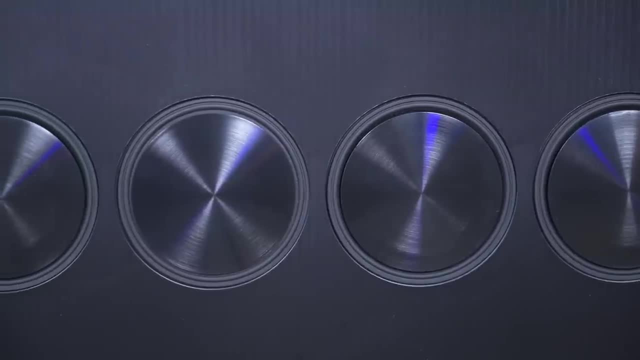 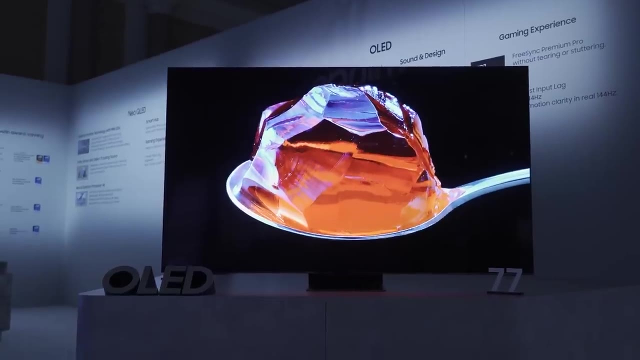 with Samsung soundbars, including wireless Dolby Atmos, surround, QSymphony sound, which uses the TV speakers along with the soundbar, for an even bigger audio experience. Then you get Samsung's remarkably effective calibration app, and I'm a big fan of Samsung's solar-powered 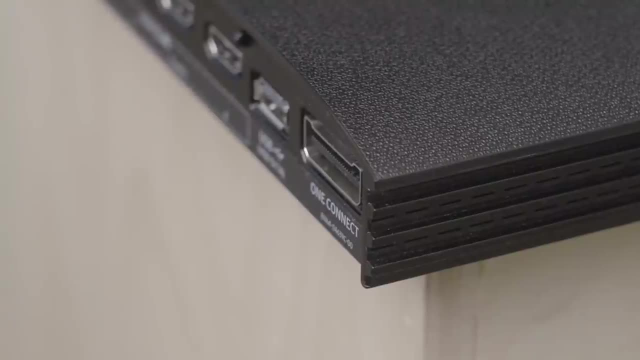 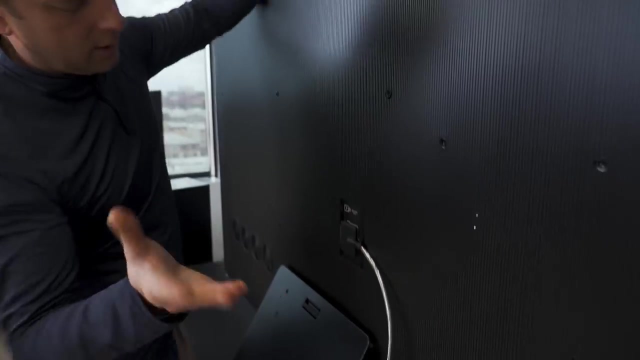 USB rechargeable remote control as well. Oh, and then there's the One Connect box too. I can't forget that This allows you to plug everything into this one box and then run one cable up to the TV. This can make wall mount installation a bit easier. 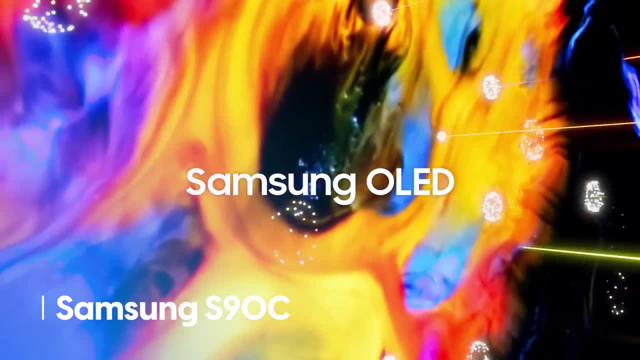 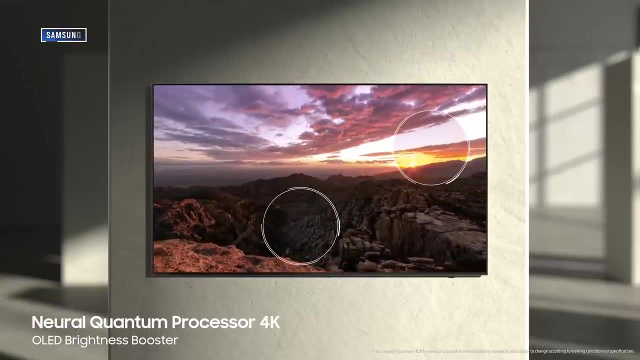 if you're gonna DIY that job. Now there's also the step-down S90C, which again gets you almost all of the performance of the S95C. it's just missing a few features like that One Connect box. Frankly, the S90C is gonna make more sense. 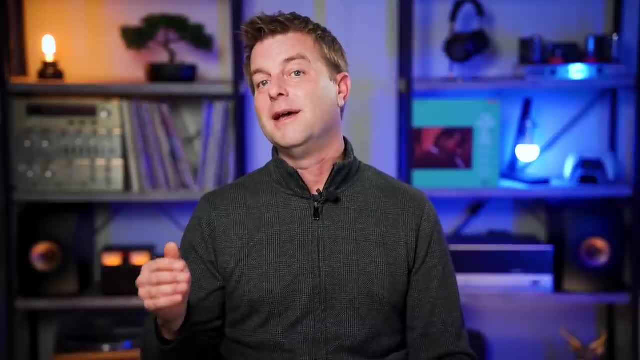 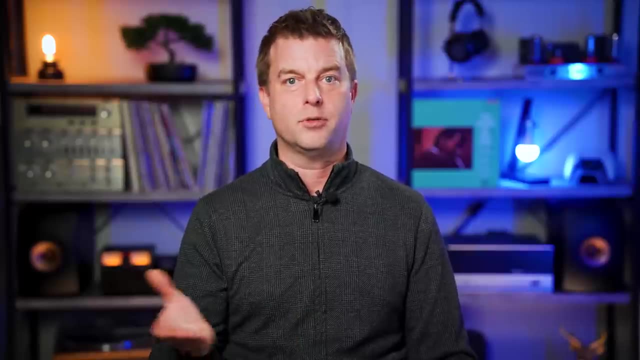 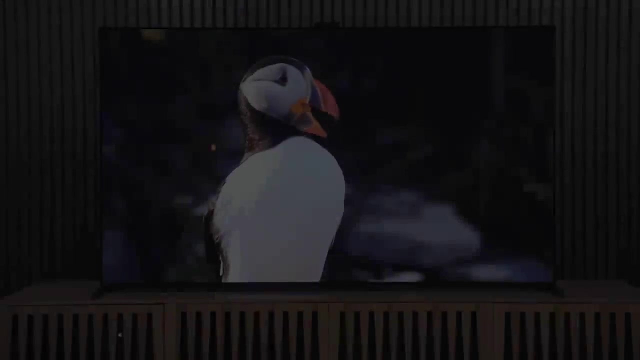 for a lot of folks who want the QD OLED picture quality but don't wanna pony up a small, small fortune, especially if you want the 77-inch model, which already commands a premium due to its size. Finally, let's talk about my favorite TV this year. 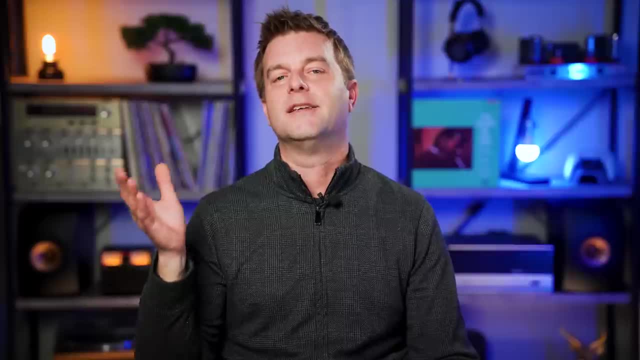 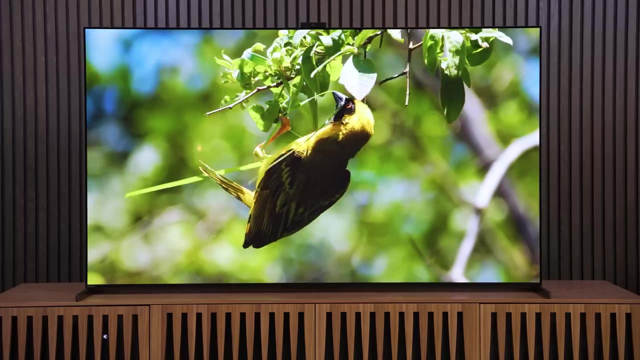 It's the Sony A95L. Folks, this TV is stunning and I just I love it so much. It's the best TV I've ever reviewed and it may stay that way through 2024,. honestly, Here's a little secret for any of my fans. 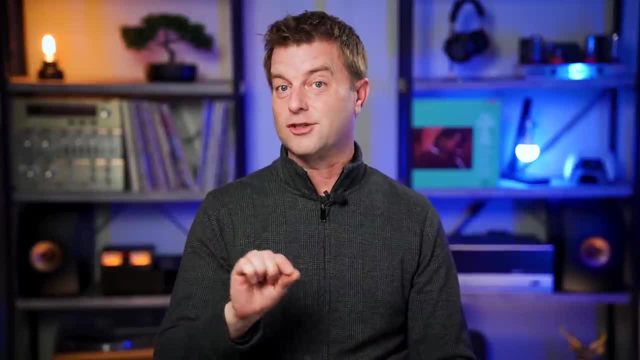 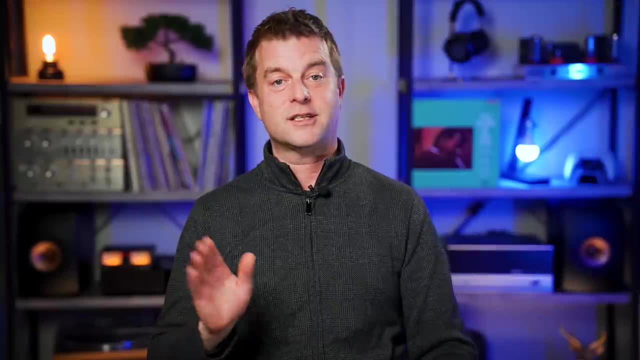 who have stuck around with me for this video. I have a feeling that the Sony A95L may not get a replacement model in 2024.. I'm not saying that for sure, It's just- let's call it- a well-informed suspicion. 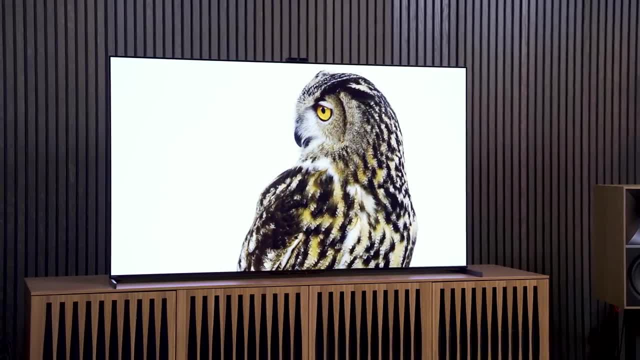 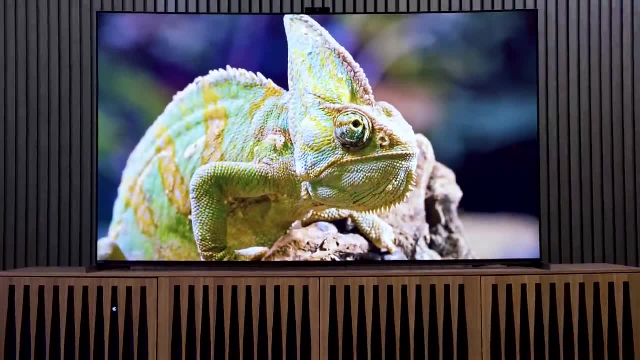 Anyway, the Sony A95L commands a real premium, and we'll talk about whether it makes more sense to buy the A95L over the other OLED TVs I put on this list in an OLED TV battle video that I'm working on right now. 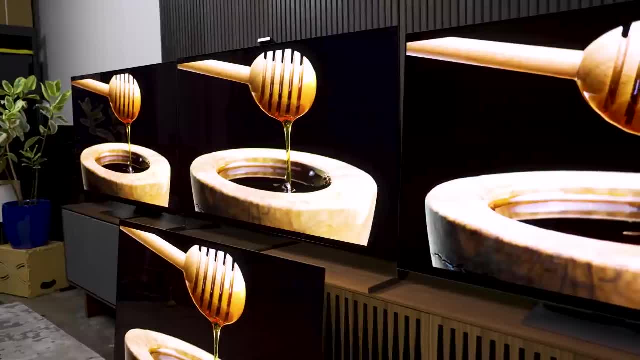 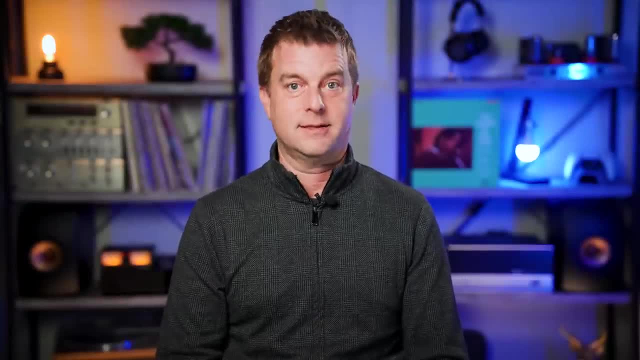 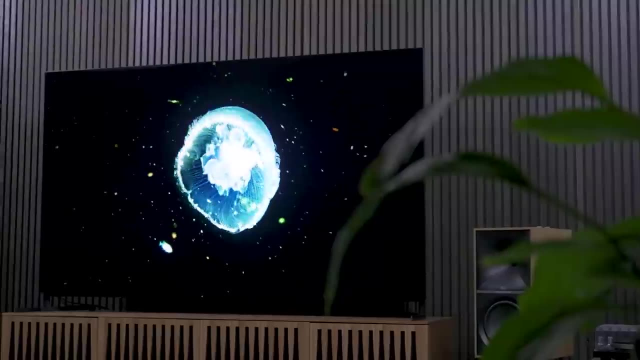 Look, there it is. I'm taking care of that in almost all of my free time. But as marginal as its superiority may be, the A95L really is the best, And once again it comes down to Sony's processing. For the same reason, I recommended the X90L and X95L. 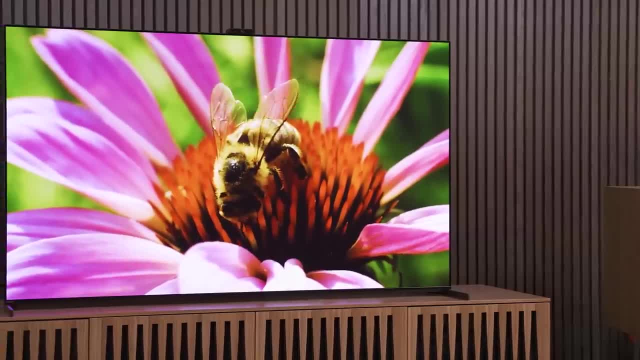 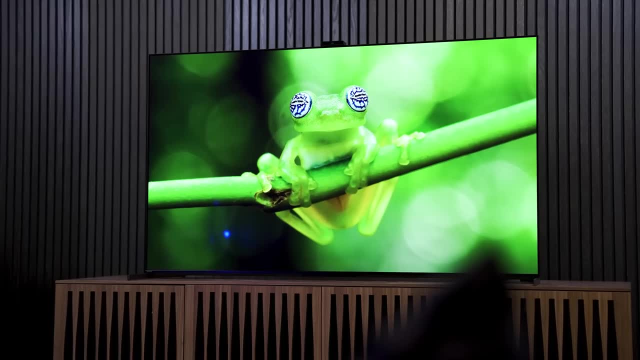 on this list earlier. the A95L comes out on top by having the most cinematic motion, the most scalable motion, smoothing a killer-looking game mode, the most accurate out-of-box performance and the best tone mapping for HDR. and the most accurate out-of-box performance and the best tone mapping for HDR. 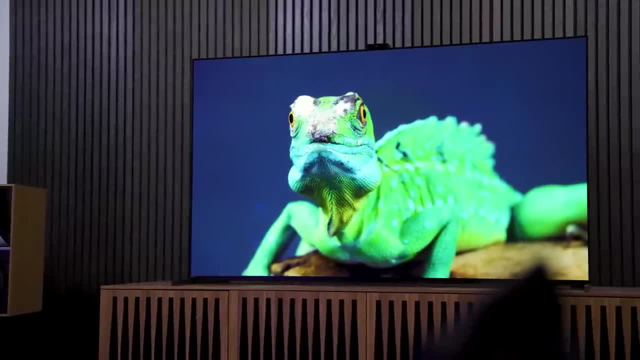 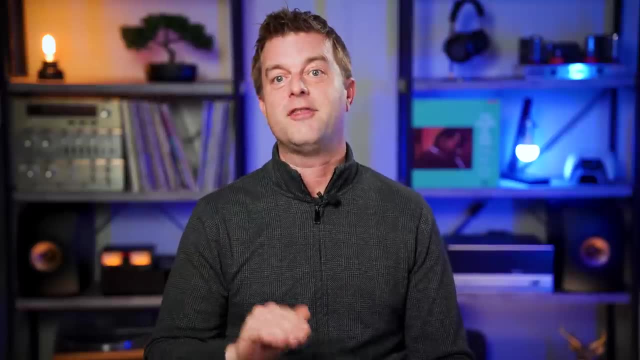 yielding these absolutely stunning images, especially for HDR content. Let me put it this way: There's not a single person to whom I've shown this TV that didn't think it was just the most beautiful-looking TV they've seen before. Am I right, Zeke? 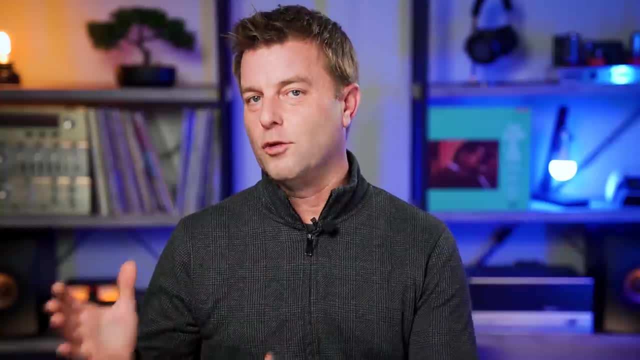 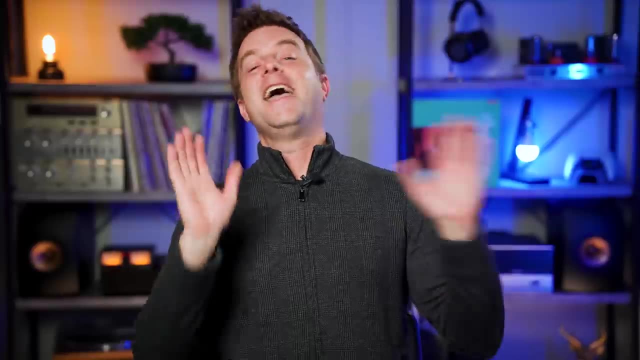 Yeah, See, Zeke knows It doesn't just deliver the wow, it delivers the whoa. I said: did I just sound like Keanu Reeves just now? Anyway, I said that in the review, I'll repeat it here. 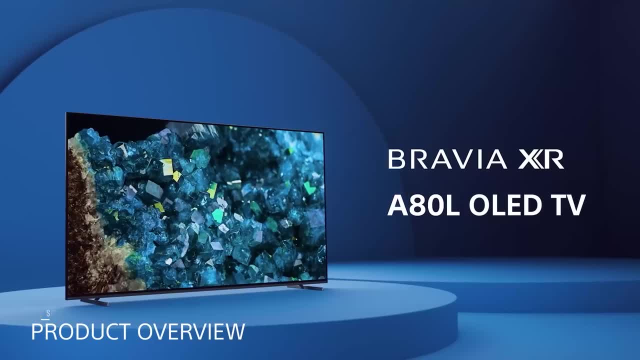 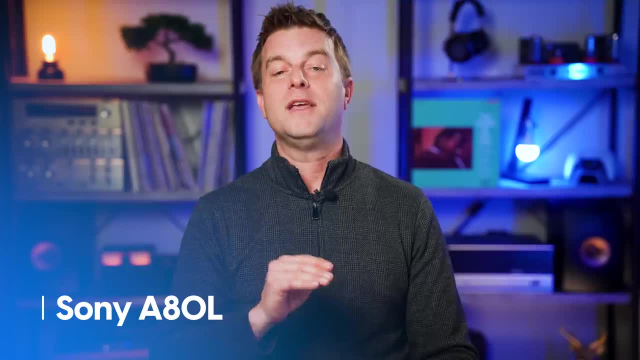 It's just the most apt description. I can't help it. Of course, Sony does have a more affordable OLED and, honestly, it's the one that makes more sense for the most people. That would be the Sony A80L. The A80L is a lot like the LG C3 I mentioned earlier. 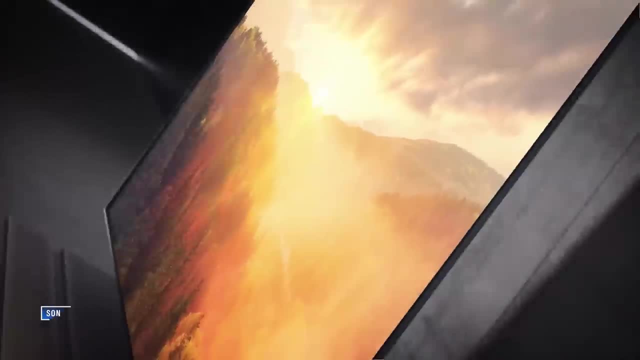 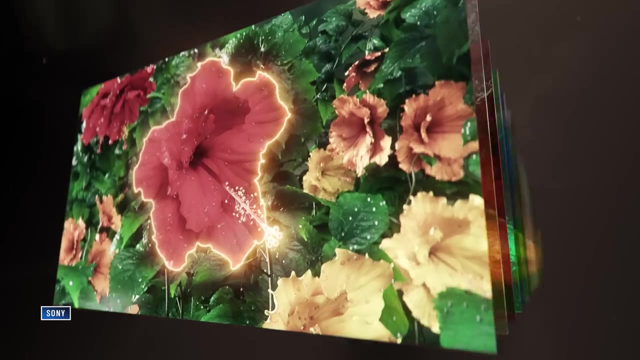 in that it is less expensive, goes up to 83 inches and offers excellent picture quality. It actually uses the same OLED panel as the LG C3, but it's got Sony's processing and Sony's take on Google TV, but it's got Sony's processing and Sony's take on Google TV. 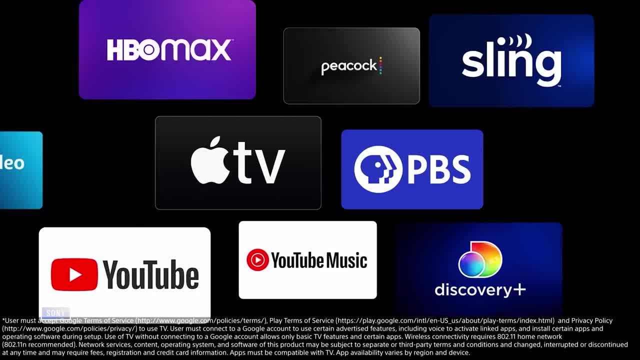 but it's got Sony's processing and Sony's take on Google TV built in, So it's just an excellent choice in its own right. That's the list, folks. Feels like a big moment for me right now. It feels good to finally weigh in.